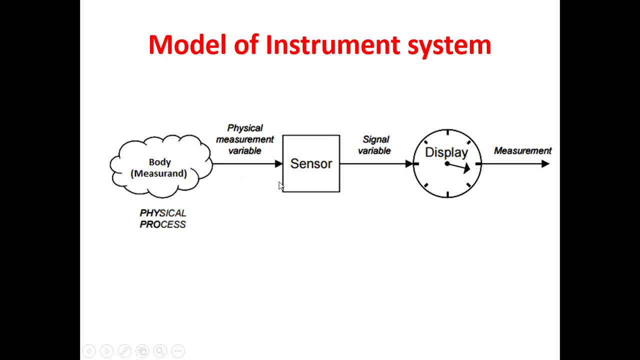 And the sensor will convert one form of energy to another form And the output is normally called as the signal variable. And this signal variable that can be used to display by the help of a display device, Or it can also be connected to a particular instrumentation system or any other kind of recording system. 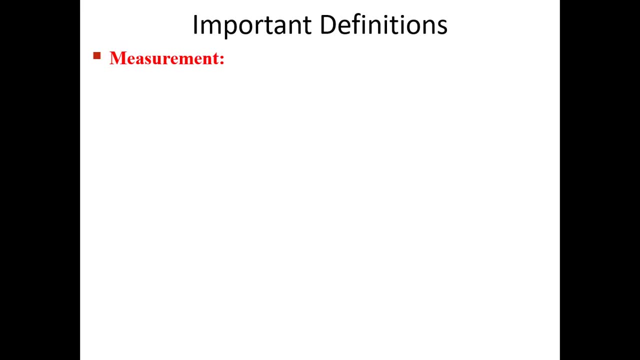 Now some of the basic definitions. it is a bit theory, but still that makes the concepts clear. So the first terminology is measurement: The process of comparing an unknown quantity with a standard of the same quantity. So it's a measurement. basically, we just want to compare the recorded reading with something of a standard quantity or a standard unit. I mean standard quantity. 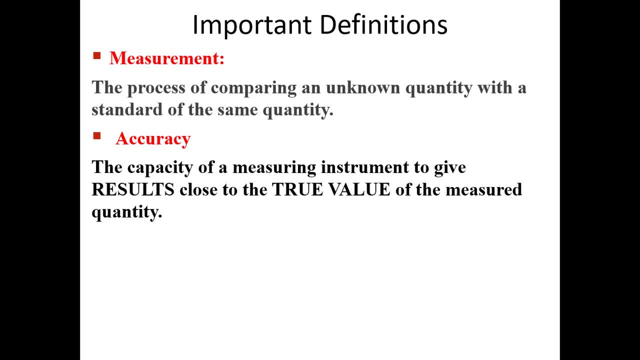 Now, the accuracy means what? How close the measured value to the true value? That is normally called as the accuracy. So the difference is Normally is referred to as the error, And basically one common type of error measurement is called the absolute error. 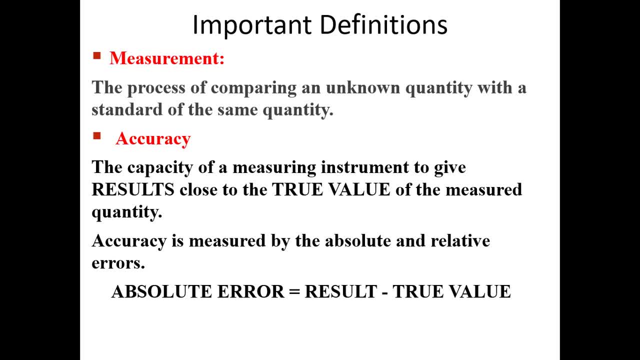 Absolute error is nothing but the distance between, or the difference between, the results and the true value. If they are close, then the absolute- I mean very close to each other, then the absolute error will be. you know less. Otherwise you know there must be some gap. 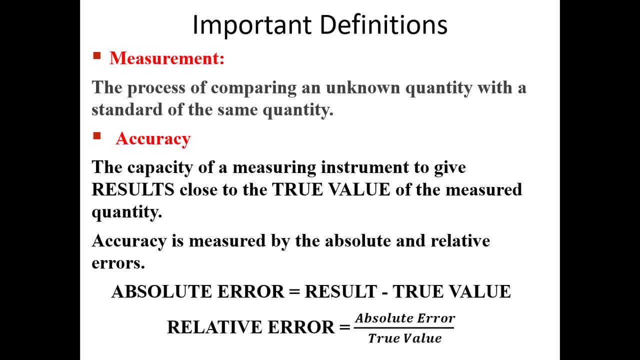 And- but most of the cases it's good to You know measure, I mean to represent the error in the with respect to something called relative error. Relative error is nothing but the absolute error If you are going to represent as a fraction of what you call the true value. 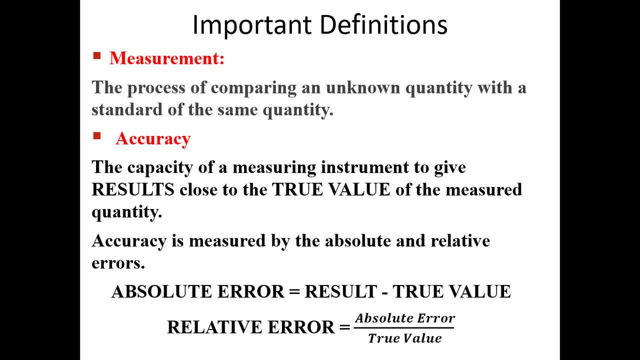 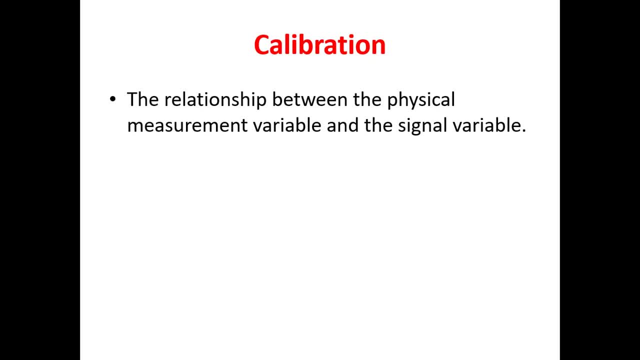 Or you are going to refer with reference to what you call the true value. So this is normally measured and referred as percentage error Calibration is a very common procedure. Normally we want to make sure that the Measured value or the instrument has to be calibrated by applying a non-physical input and recording the response of the system. 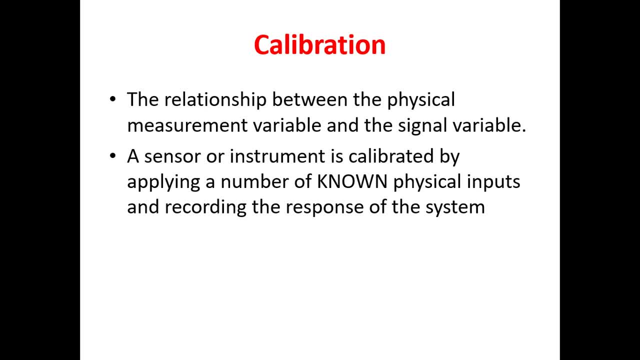 So, basically, calibration means what we want: to make sure that our recorder reading of the obtained reading is close to the what you call the standard value, Right. So how can you do that? You know, we can do by calibrating the instrument, by applying a non-value to the instrument and the reading. 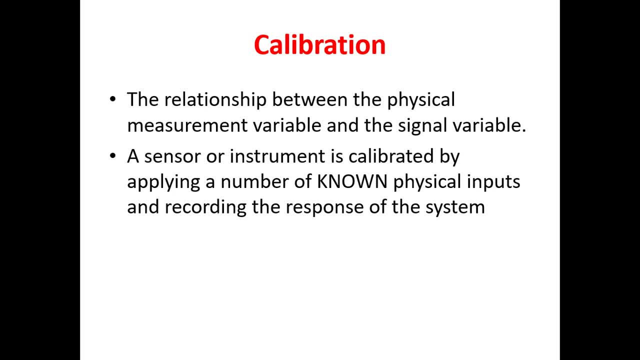 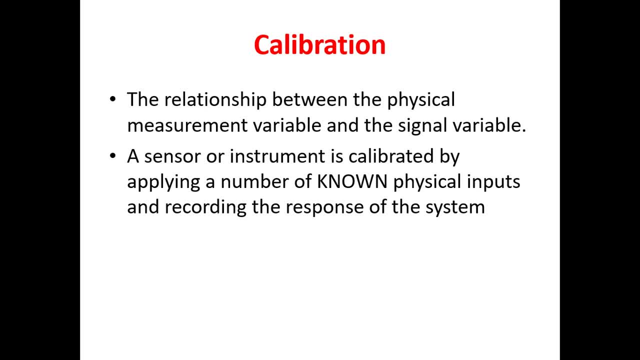 Right, Right, Right, Right, Right, Right. So calibration is a very important step, especially in medical equipment, in laboratory instruments. Make sure that the system to be calibrated for a non-parameter and we want to make sure that the observed reading is within a specified error limit. 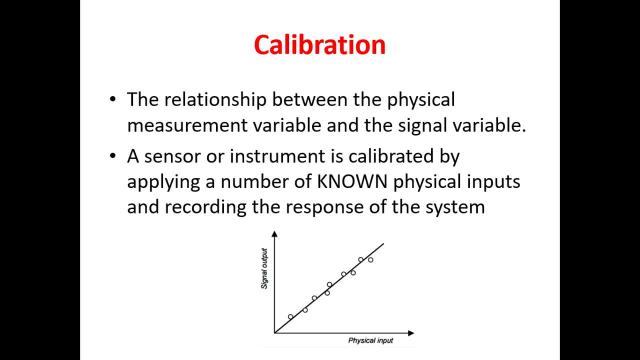 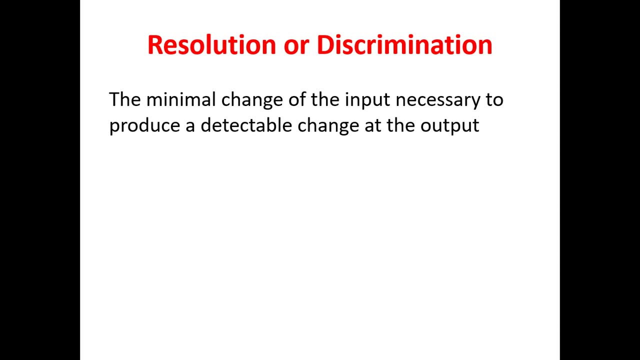 So that is basically called as the calibration. Now another important term is called the resolution is also called discrimination. It is a minimal change of the input necessary to produce a noticeable change at the output. This is basically called as a resolution. So how sensitive the resolution is very similar to something called the sensitivity, a minimal. 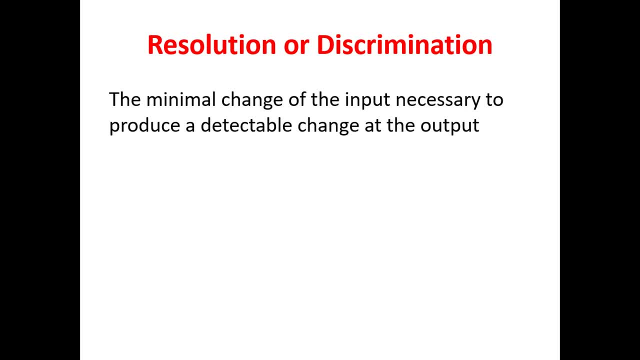 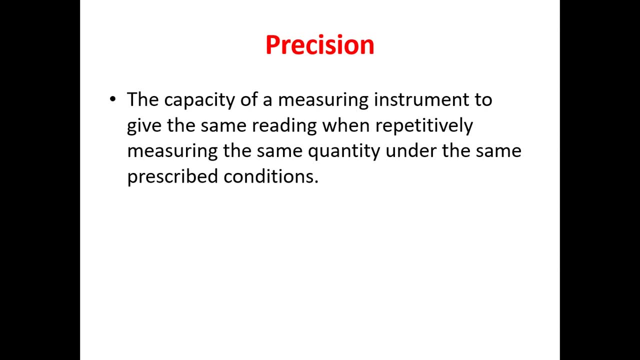 change of the input that is necessary to produce a noticeable change in the output. So the meaning is our system should be capable of detecting a small change in the input. That is the capacity, or that is the capability of an instrument. Now another terminology is called the position. 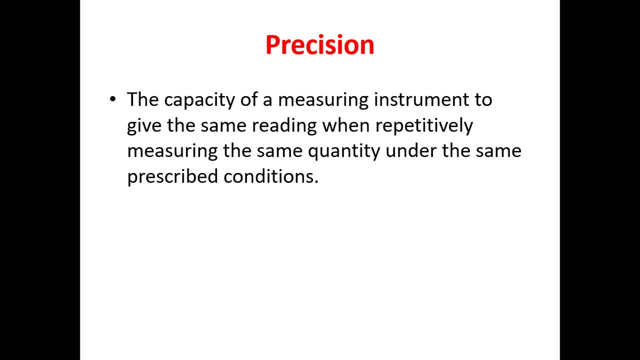 The capacity of measuring instrument to give the same reading when repetitively measuring the same quantity under the same prescribed conditions. Suppose, if you are going to repeat the same experiment within the same environment, the same systems, Same equipment set up, same experiment set up. if you are going to repeat the experiment. 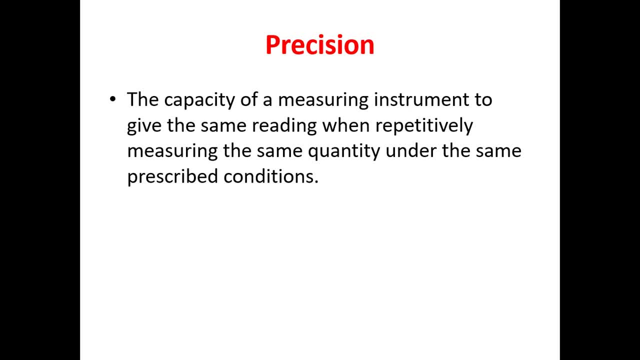 again and again with short interval of time, then this is: if you are getting this similar reading, then we can say that this is a precision. actually, Now, the precision implies the agreement between the successive reading, not closeness to the true value, but the reading. whatever reading we are getting, we want to get the consistent. 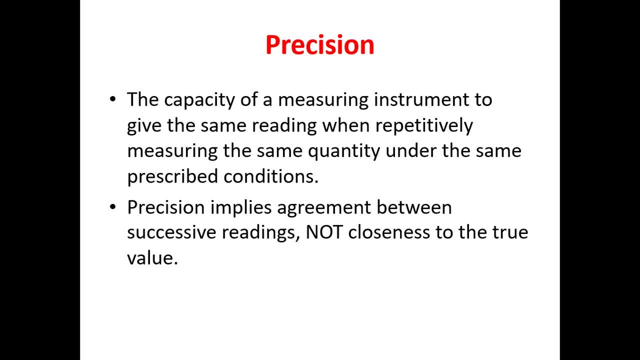 reading again and again. It may be very- I mean it may be very- different. It may be different from what you call the actual or the true value. But whatever value you observe it, that value will be repeating again and again. So this shows the precision. 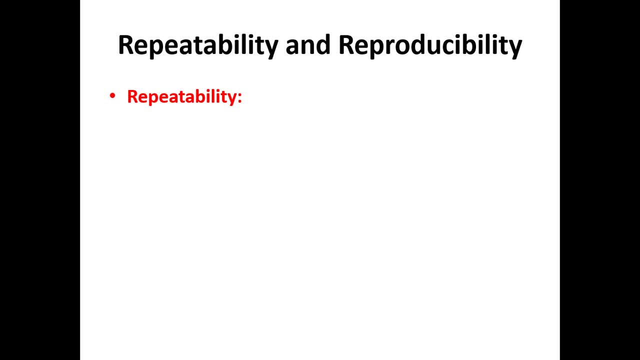 Repeatability and reproducibility, you know, are the two concepts which are very, very, you know, much related to what you call precision. In both case, you know, we are using the precision terminology. Repeatability means what? 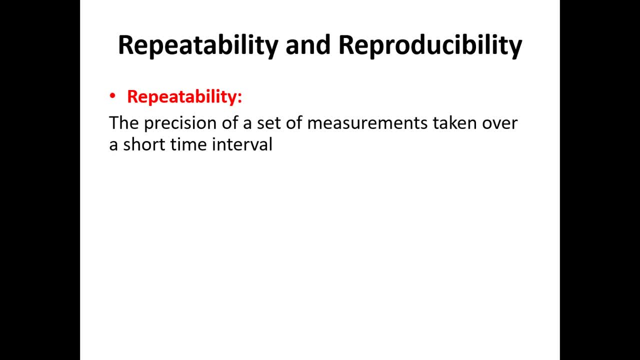 The precision of a set of measurements taken over a short period- you know interval of time- which means that we are going to repeat the exercise or the experiments- you know with some numbers or you know with some parameters- But that the experiment interval is going to be as short as possible. 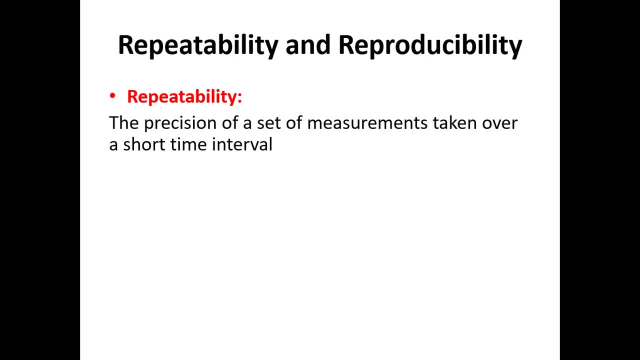 So if you are going to repeat the exercise, you know, within a very short period of time, then if you can reproduce- I mean, if you can, you know- get the same reading again and again, then it is called a repeatable right. 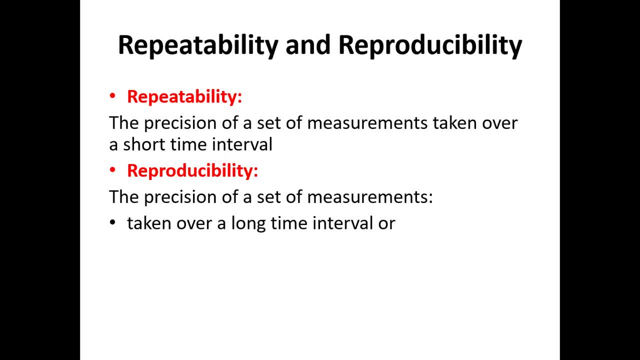 And reproducibility, on the other hand, is talking about if you are going to do an experiment which is for a long interval of time- the time is, like you know, really long interval of time- and also it is performed by different operators. they are doing the experiment. 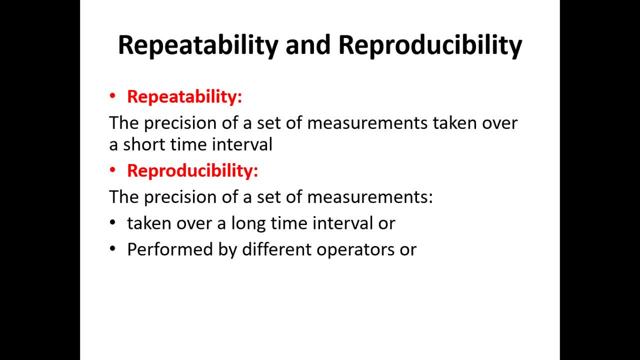 you know, You know different operator and also with different instruments. you know, we are repeating the experiment with a different instrument and also maybe with different laboratories, And if you can get the similar reading, then we can say that this particular you know. 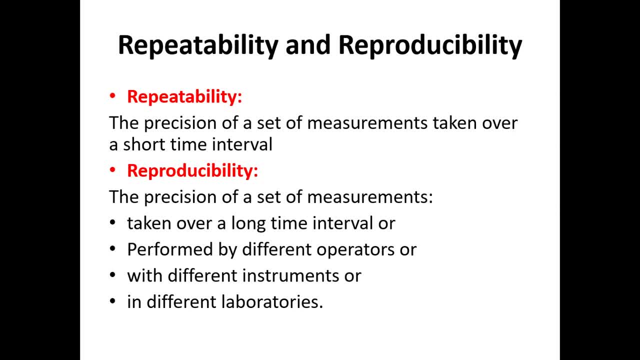 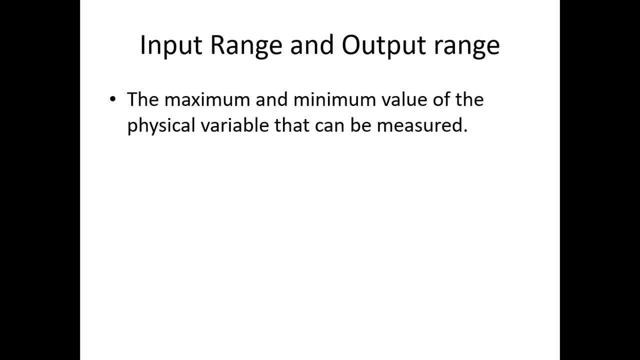 experiment is said to be, or this particular, you know trial, is going to be reproducible. okay, So there is a difference between repeatability and reproducibility. okay, Now, input and output range are indicating the maximum and minimum value of the physical. 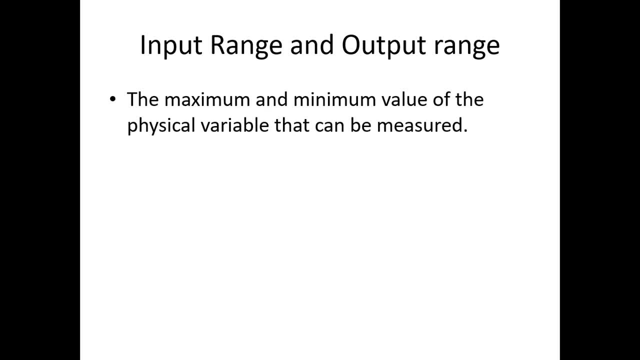 variable That can be measured. you know The maximum and minimum value of physical variable that can be measured. So that range of the maximum and minimum that is basically called as the input as well as the output range. okay, This sensitivity already we have discussed and sensitivity, you know that it is a change. 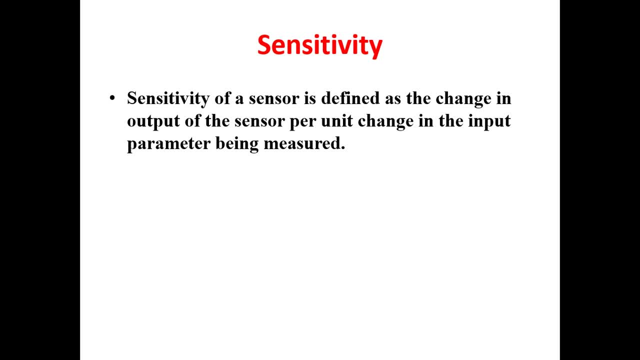 of the output of a sensor per unit change in the, you know, input parameter that is being measured, So higher the sensitivity, which means you know this is like a ratio: we have numerator that is the output and denominator is the input. 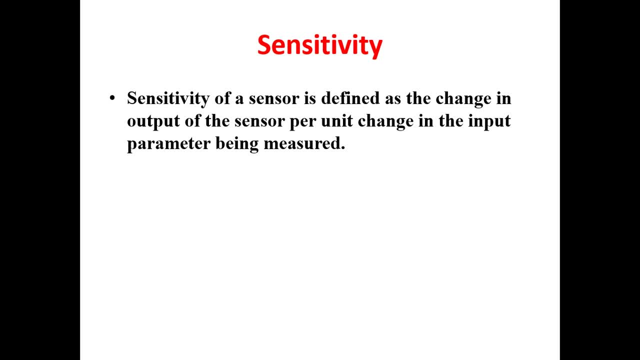 And if you have an IR ratio which means that the sensitivity is higher, which means that for every small change in the input there will be, you know, a large change in the output, okay, There is something called sensitivity here. Now another term is called linearity. 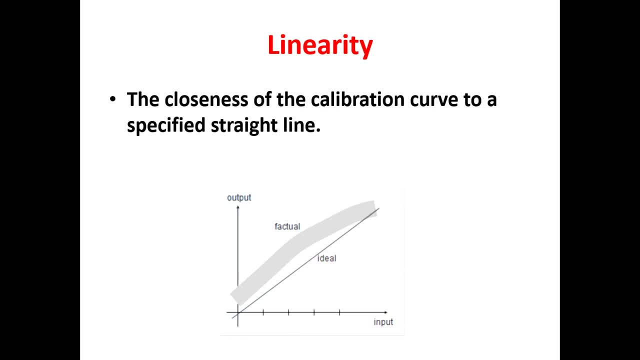 Linearity means what? the closeness of the calibration curve to a specified straight line here. okay, So this is basically say cal, or the calibration graph, This is an ideal graph And you know how close in the actual, the value to what you call the ideal calibration. 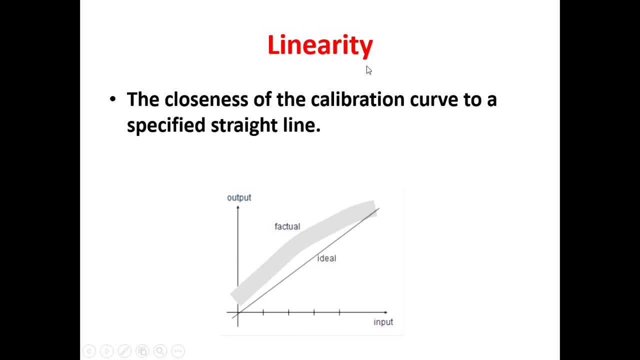 graph, then that is basically called as the linearity. okay, Linearity is also one of the very important relation And hysteresis means the difference between two output value that corresponds to the same input. okay, which means that we are going to repeat the same exercise again, because 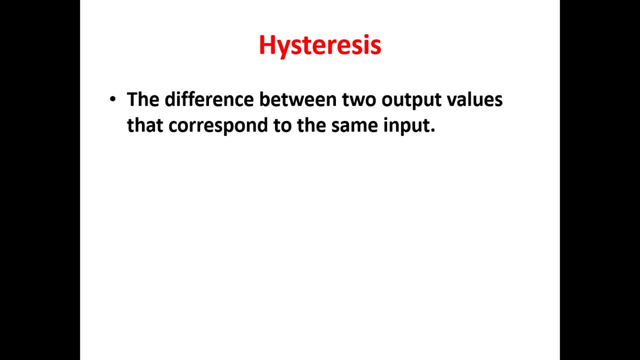 of the…. And also sometimes we can do a cyclic logarithm. Okay, Loading in the sense, for if you are applying a positive quantity, then if you are, then we are applying a negative quantity. right, Then try to find out. you know the difference. you know if you are going to get in the output. 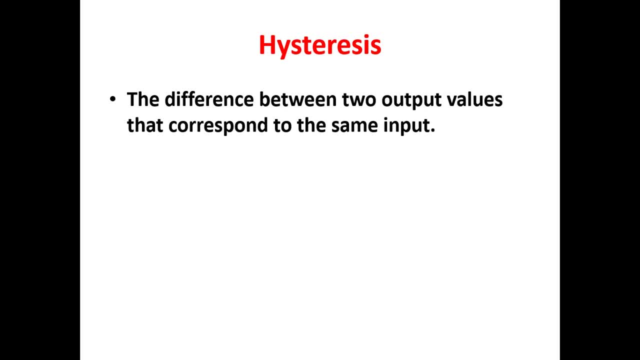 when we are, you know feeding what you call signals, or the quantities or the measurements. you know measurements with. you know what you call different, you know amplitudes, I mean especially in a sign also, So the…. 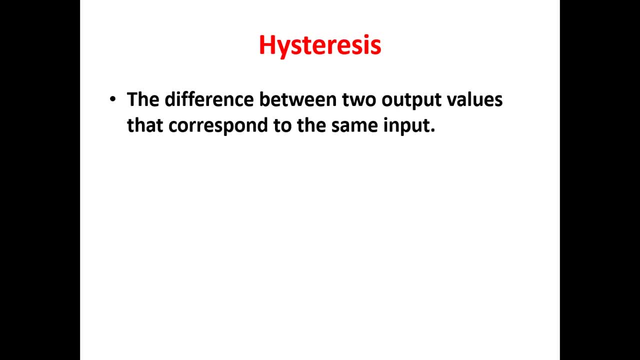 The… The… The… So the… Th percent result is 100, which means what We are going to apply positive and we are applying negative. So we are going to apply cyclic load or the cyclic- I mean measurements- to the instrumentation. 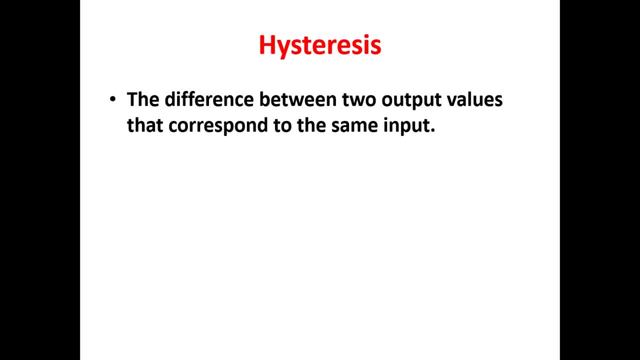 system and try to find out, you know, if there is any change in the output. That is basically called as the hysteresis. Okay, Now this particular graph indicate the you know the difference between precision and what you call the accuracy. 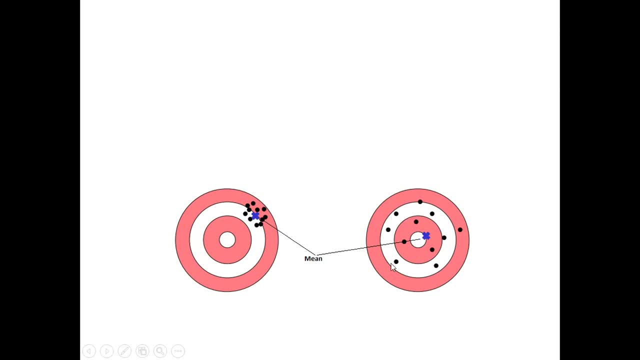 Here you can find that this is the target point And you know these all black dots indicate that most of these you know shoot are. you know shots are happening exactly like and and so on. It is very important, Okay. 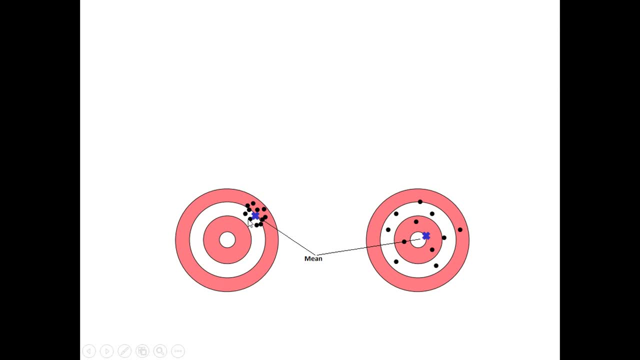 around the target point here, but in this case we can find that you know, these black dots are are all concentrated, you know, at one particular point, but even though there, it is far from what you call the target point, but it is very highly precise. so this is highly precise, whereas this: 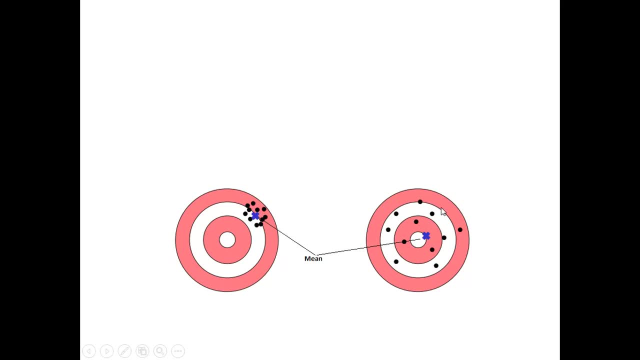 is, you know, highly accurate? i mean not, can see in a accurate but not accurate. but it's accurate okay, but this is talking about highly precise okay. so this point: indicate the mean value. so if you see here the mean value of what you call the all the shots, you know will be something very 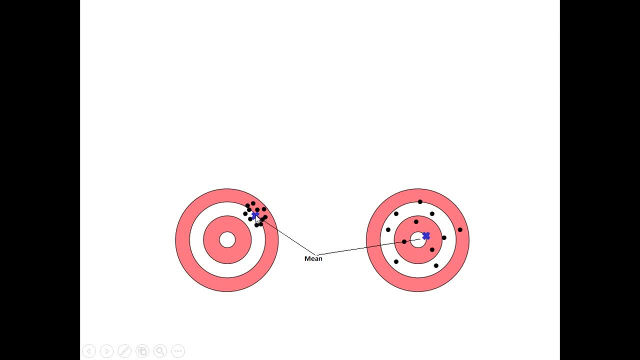 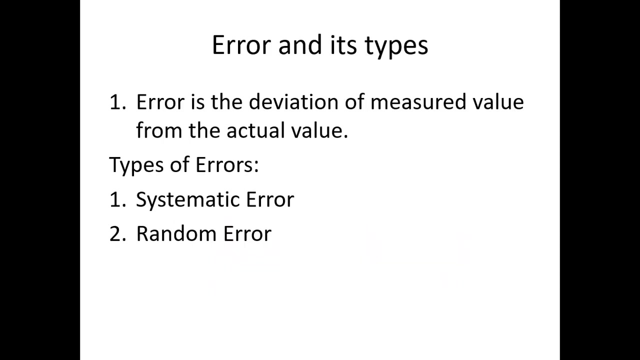 close to what you call the target value, but the mean value somewhere here. actually also, this is the difference between precision and accuracy. with reference to, you know some diagram- i mean in a diagrammatic way- now in this slide they're going to discuss about, you know the, the error, and 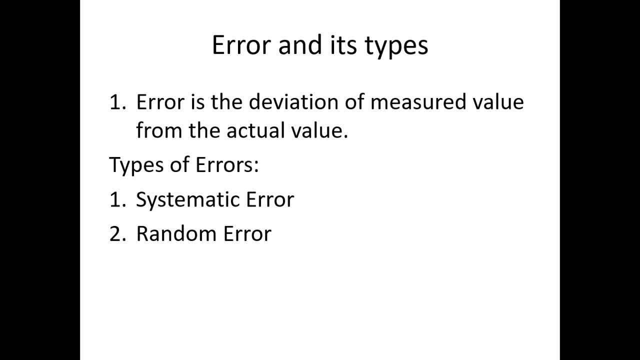 you know, then, the different you know the error and you know the different different types of errors here. so the errors are is basically the deviation that is measured between the measured value to, you know, to the actual value or from the actual value. type of the errors are systematic error and random errors. systematic errors are result of many you. 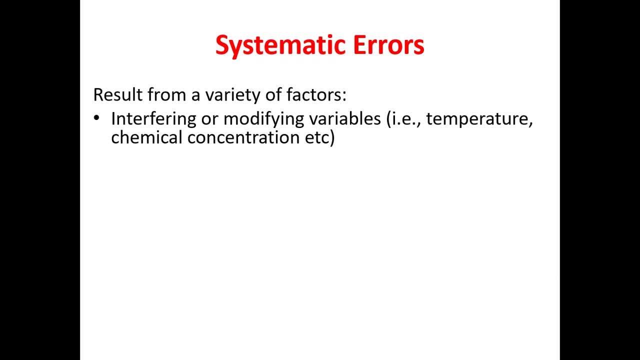 know variety of factors and could be interfering or modifying variables such as the ambient, you know working conditions such as the temperature, pressure, chemical concentration, etc. a system which is designed for a particular environment probably wont work. you know with an. you know a different. you know atmosphere or different. 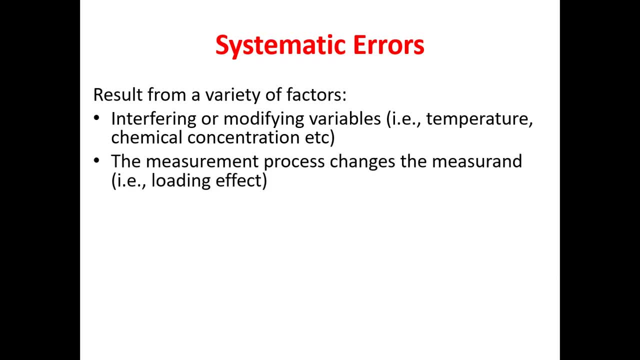 no working conditions. ok, so this is one of the systematic error. the measurement process changes, you know the measurement, which means that if you are applying heavy loads- ok and tiny- you know tiny loads and heavy loads- this will also create, you know, some kind of you know errors. and the transmission process changes the signal, for example the. 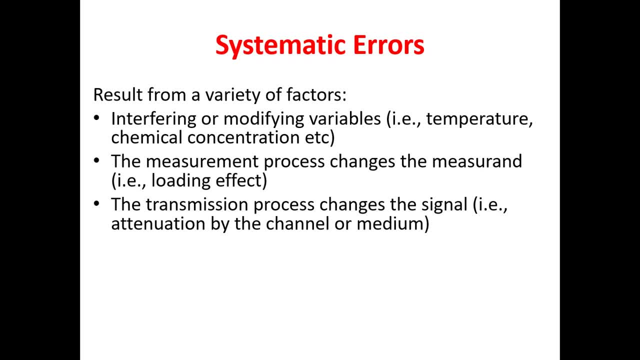 transmission process changes the signal. for example, the signal may be affected largely by the surrounding noise, and especially when you are transmitting the measured signals. in such cases, the accuracy of the system will be depending upon the noise. This is also called the signal to noise ratio of the system. 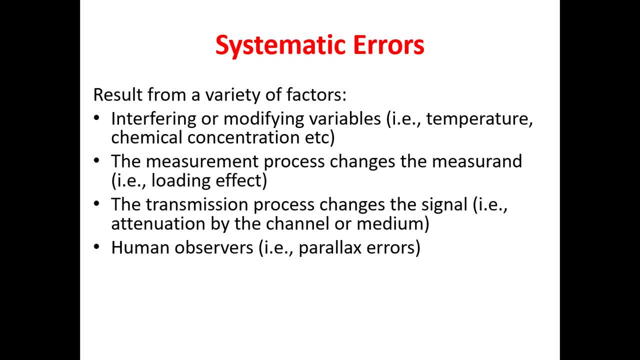 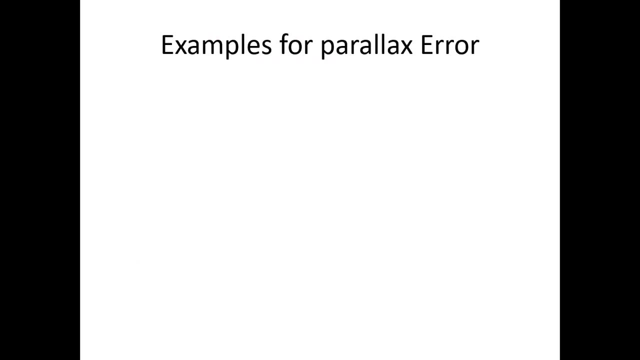 Now, the human observers is also one of the points which is normally referred to as parallax error, And parallax error is an error just because of the position or the orientation of the observer. So I am going to show you some example here. So, for example, in this particular case, here. so we have three scenarios, and this is the. 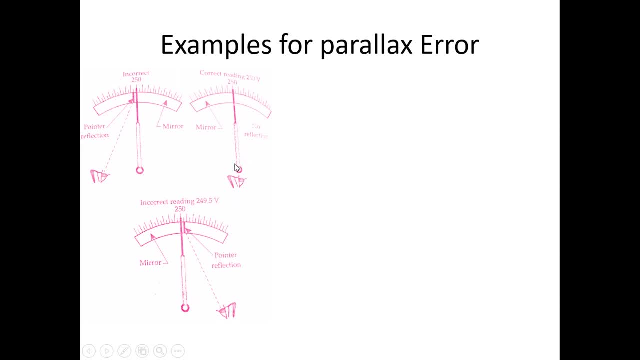 actual scenario where the observer is exactly aligned to the pointer. whereas this is the observer is located on the left side and this is on the right side. In both left and right you can find some change. In the case of left, The reading is you have a higher reading, whereas if the observer is on the left side. 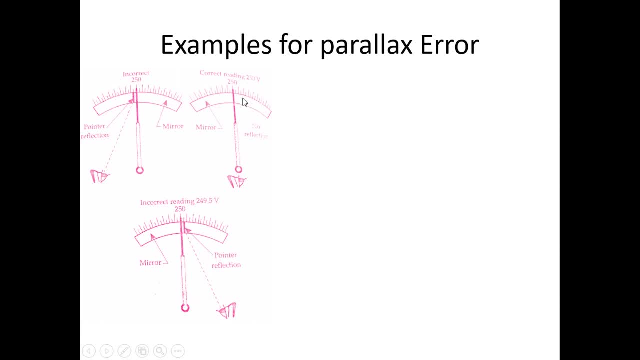 you know you have a lower reading, Okay, But the actual value is supposed to be 250, so it is slightly. in the case of left side, it is slightly positive, I mean slightly above 250, and when it is left right side, it is slightly, you know, negative. 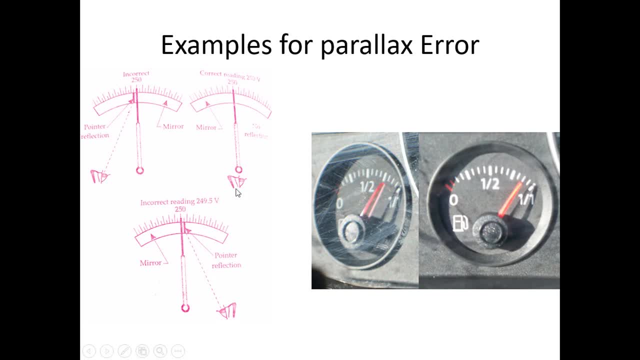 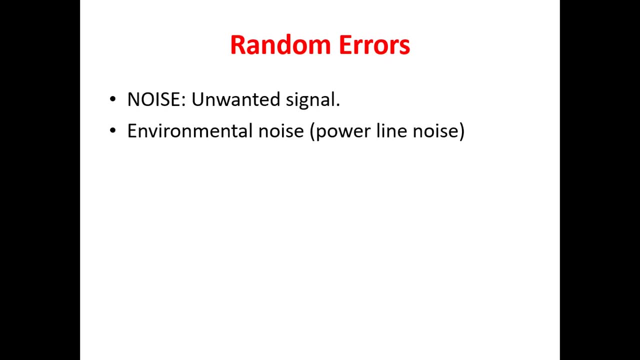 I mean below 250.. The same thing you can observe in cars and you know other, what you call analog instruments, Random errors. So these are some noise or unwanted signals whose origin you know we cannot define. There are also some environmental noises, So that's why always it is better to keep you know: signal to noise ratio is always far. 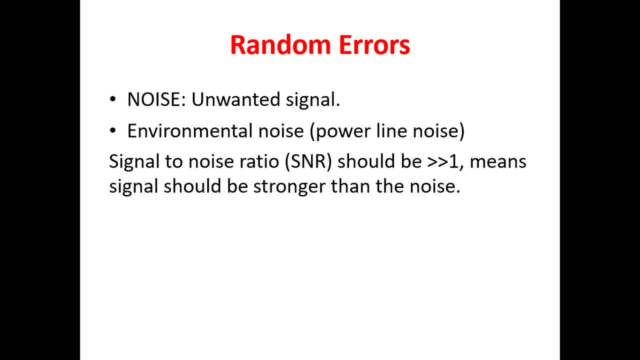 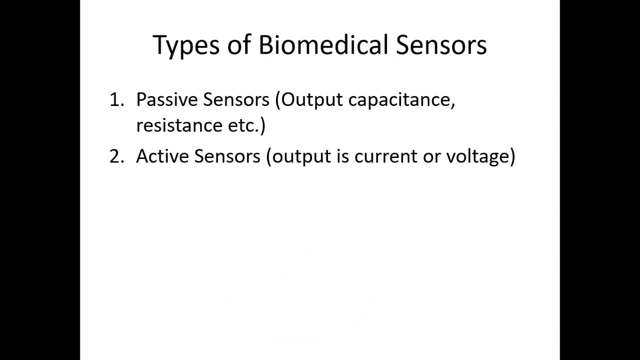 far greater than one, which means that signal should be stronger than the noise. here Now type of biomedical sensors. The sensors are mostly classified into passive sensors and active sensor, depending upon the output, Whether they are in an active form or passive form. So if it is a passive form, which means that the output will be in the form of capacitance, 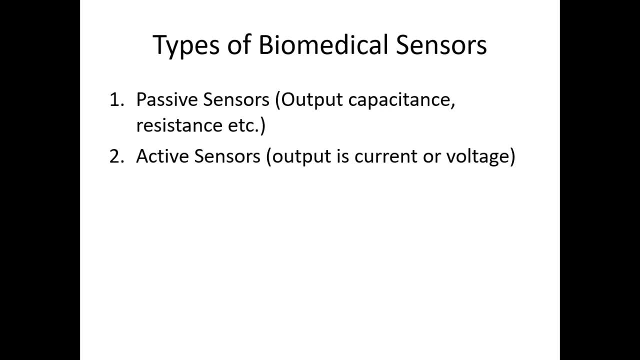 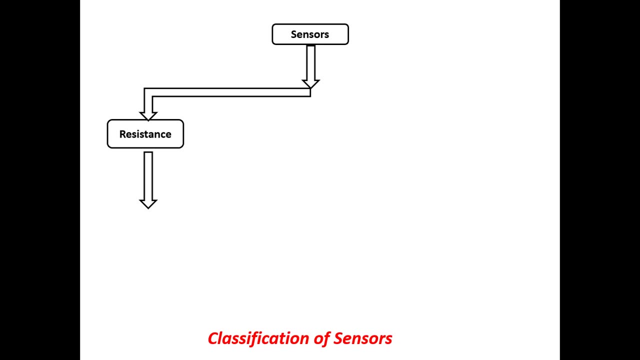 resistance, inductance, etc. Whereas in the case of active sensors the output is either in the form of current or voltage. Now let's look at the main broad classification of the sensors. The sensors are mostly classified based on the basic, the principle by which it works. 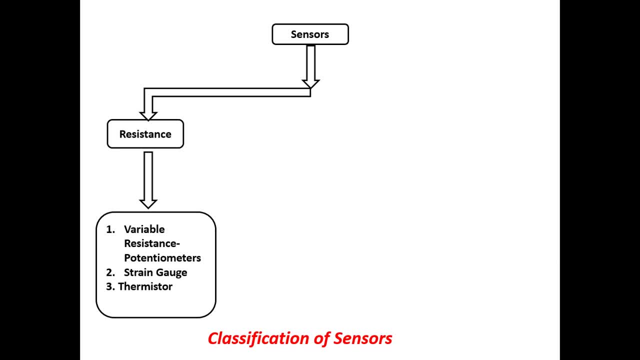 The first thing is called the resistance. The resistance sensors are classified into various types: Variable resistances. This is also called the potentiometers, Strain gauge sensors. and then we have the thermistors, The temperature resistance or the resistance temperature detectors. 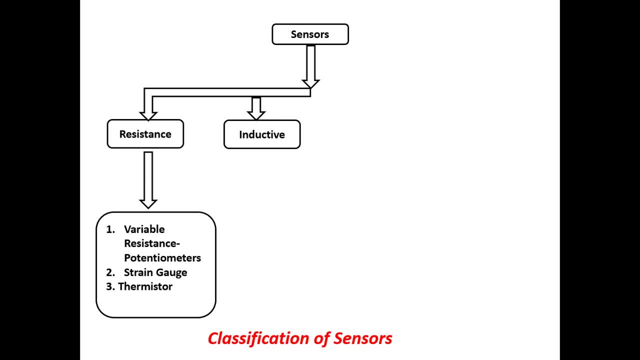 Now the other type of classification is the inductive sensor. Here the principle is inductance. So there is the physical quantity is going to change the inductance of the material. So in that we have linear variable differential voltage. you know, linear variable differential. 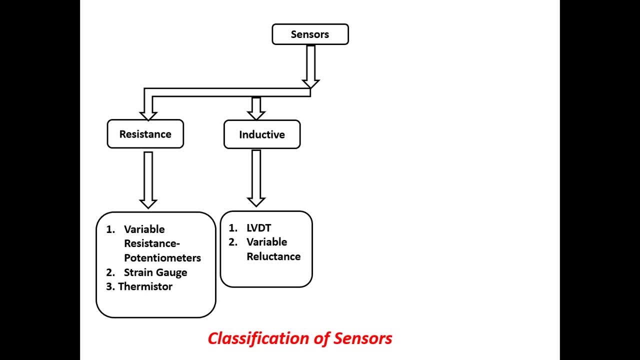 transformer transducer. It is an inductive type of transducer. Then also we have something called variable reluctance, you know reluctance transducers, which I am going to discuss here. So the next type of sensors are the capacitive sensors. Here the physical quantity that is being measured is going to make some changes on the capacitive. 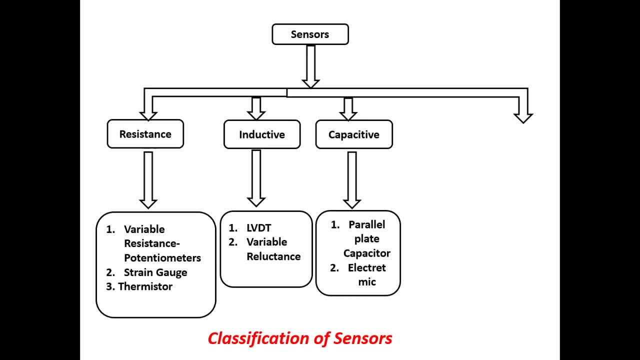 parameters, Okay, And here we have parallel plate capacitors, We have the electric mic, and these are the different type of sensors which we are going to discuss in detail Now. the other type of sensors are photo sensors. Here, these sensors are used for transforming photo or the light into electricity. 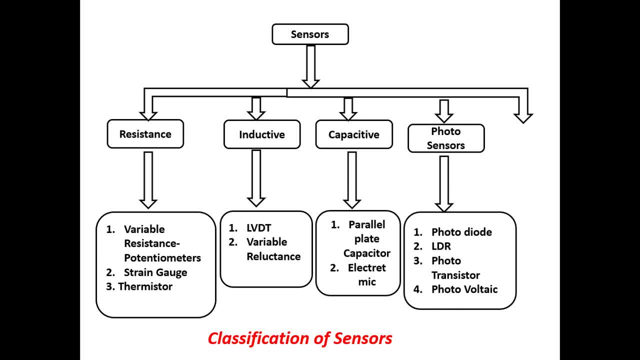 Okay, There are many type of sensors available, which include the, you know, photo diodes, the light dependent resistor, which we also call as LDR, Photo transistors, photo voltaic cells, and so on. Same way, there are other type of sensors which are very common. 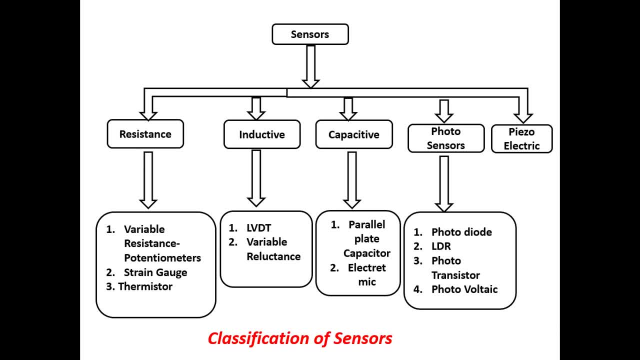 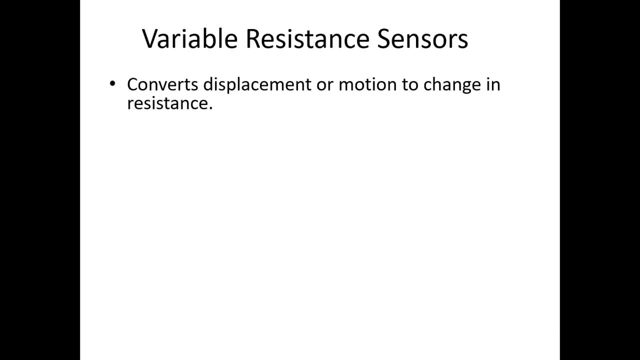 And very you know potential sensors. they are called the piezoelectric sensors. They are capable of transforming the electrical signals into mechanical vibrations and vice versa. Now let us see the variable resistance type of sensors which convert the displacement or motion into resistance changes. 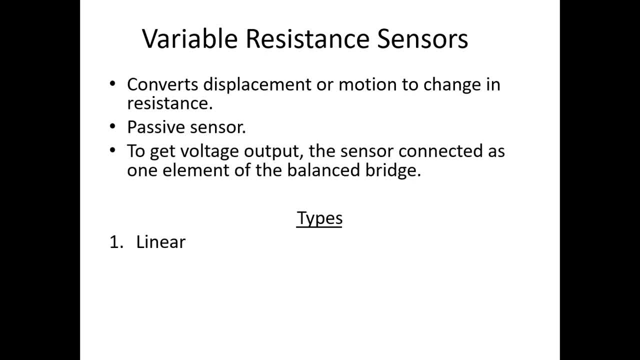 Okay, Now there are different types are available depending upon- you know the use There are. I mean depending upon the input as well. So we have linear type and angular type. Linear type- you can see from this particular diagram- is a linear type where you will find. 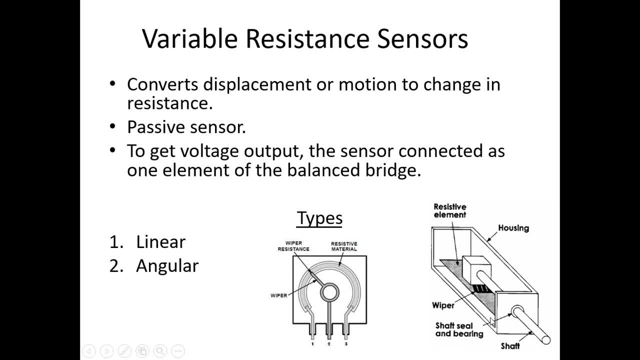 there is a resistive element where it is like you know, you know like a linear plate. Okay, You can find there is a you know a plate here and over which what you know there is a move part is going to move here. Okay, 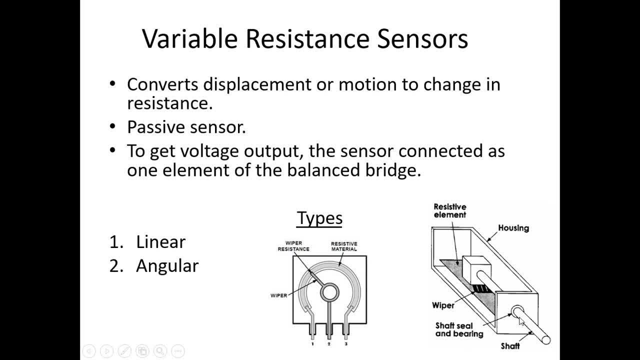 So we have a wiper, which is attached, And we have a shaft, And we have a shaft here, And this shaft will be moving along the what you call the resistive element, And resistive element is, you know, to be, in the form of what you call, you know, rectangular. 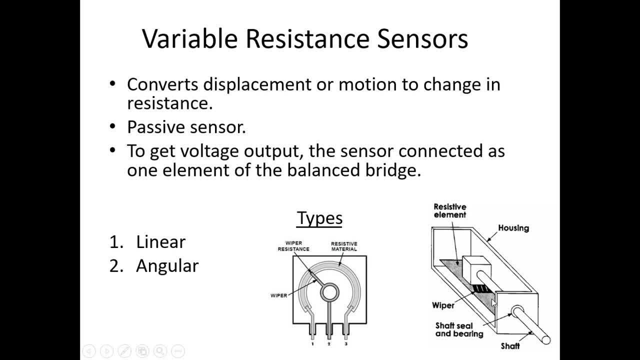 you know plate. So here what is going to happen? you know the linear motion, that linear motion that can be converted, or the linear displacement that can be converted into change in the resistance. here, On the other hand, if you see, here this is an angular, you know sensors, or the angular. 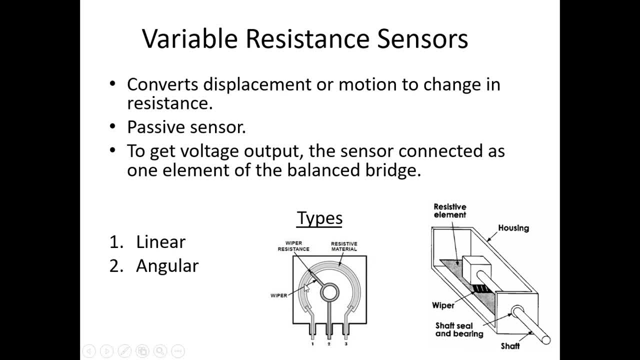 resistance sensor where the change that is going to takes place. you know the physical input is supposed to be in the angular motion And this angular motion is converted into electrical resistance here. So both you know these type of sensors are belongs to the passive, because the reason 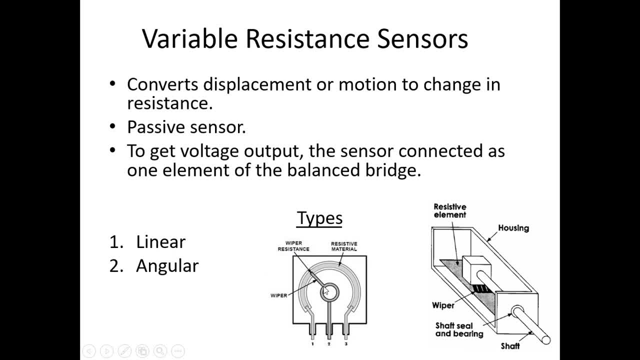 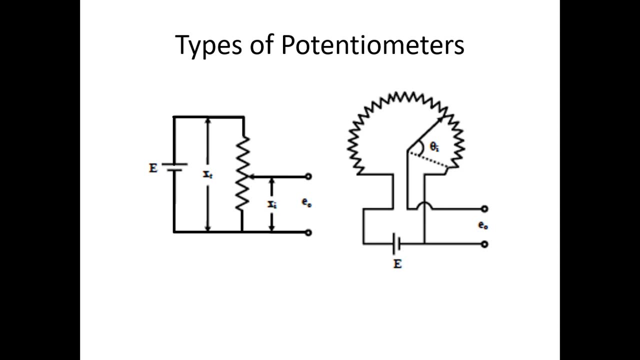 is the input, is what you call the physical displacement right, either angular or linear, but the output is in the form of resistance. Now this particular linear sensors, I mean the resistance sensors that can be converted into an active, you know, by adding some bias over here. 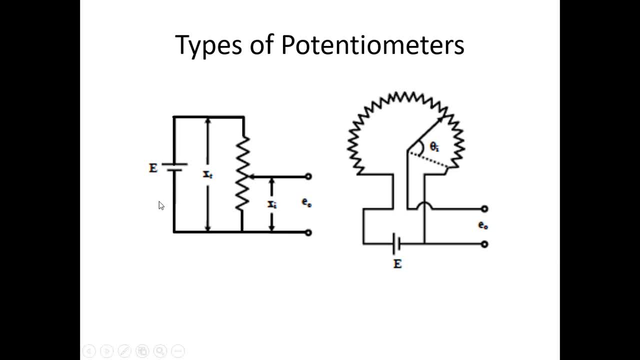 So by adding by some bias voltage, you know E we can get the change in the in the resistance sensor due to the physical movement into what you call electrical signals, I mean into the output voltage. So here it is simply acting as a potential divider where the input resistance of the 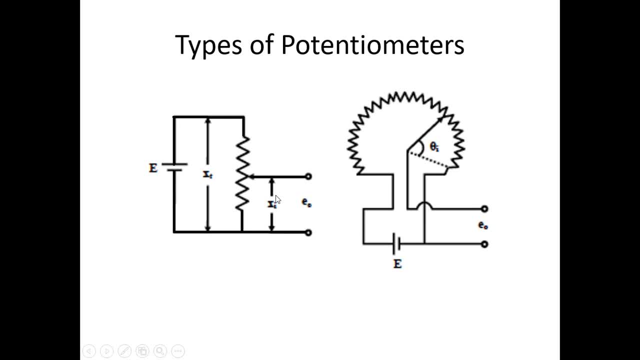 the input stage will be Xt, the total resistance, whereas this is supposed to be Xi, And this Xi is depend upon the, you know, physical motion or the physical displacement. So this output voltage will be a fraction of what you call the input voltage, and the maximum voltage we can get here is E and the minimum voltage we can get it is, you know. 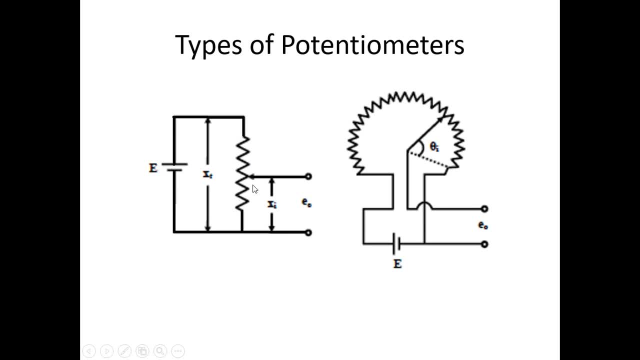 it is like zero and, depending upon the position you can have, you know any, what you call voltage, and that is nothing but a fraction. So normally the fraction is, you know, ranging from zero until one. So you may find any number from any voltage, from zero until you know one. 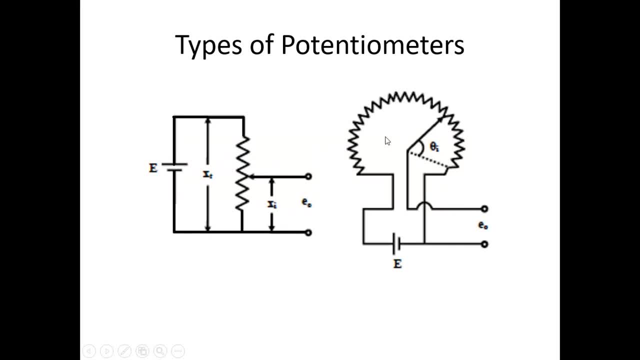 That can be obtained here. Now, in this particular case, you know we are talking about the same principle, but it is working in an angular way. the resistance orientation is in an angular, you know fashion- and again, we are using a bias voltage in order to get the output. 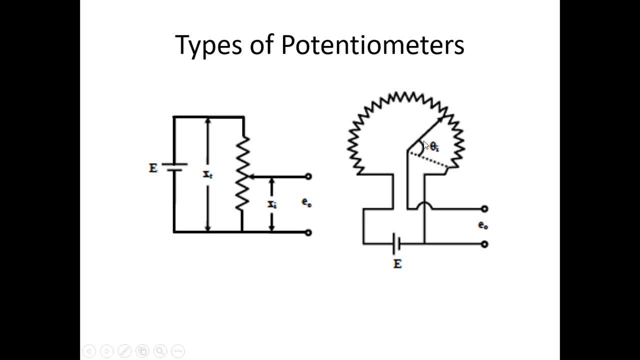 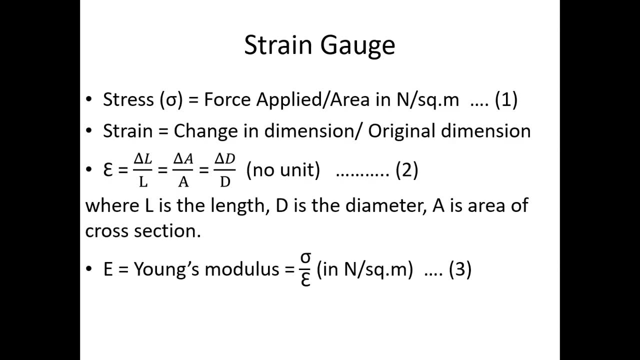 So here the input will be theta, the angle, angular displacement, and that is going to change into the output voltage here. So now the next type of sensor is the strain gauge. It is also belongs to the resistance variable resistance sensor, and this sensor is capable of transforming strain into electrical resistance. 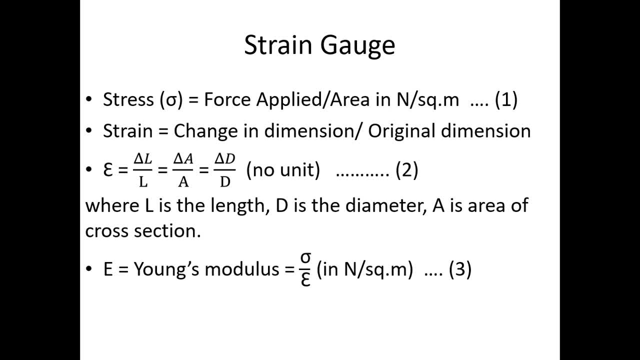 So before we discuss into the structural details of the strain gauge, we will have, you know, some basic understanding about what is stress and strength. you know stress and strain. So, basically, stress is indicated by sigma. It is nothing but the force applied in Newton, you know, per inch. 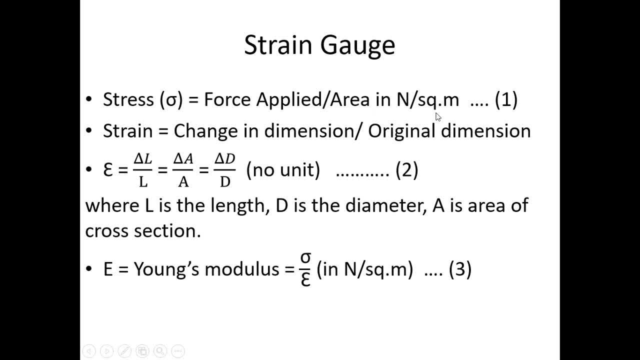 It is divided by area. okay, Normally unit is in Newton per square meters. So the force applied divided by area is basically called as the stress, So the corresponding. when you apply a force on a particular material, correct or load on a material, the material try to stress or the material try to withstand, you know the applied. 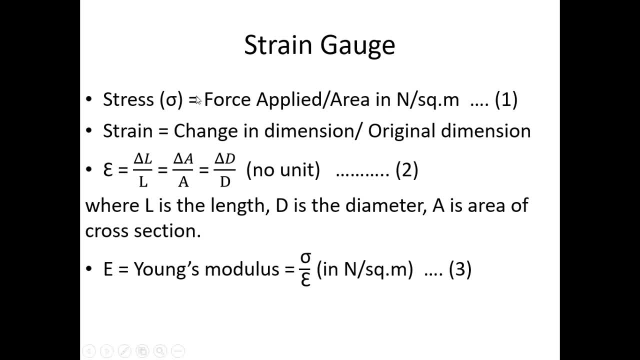 force, That particular internal force, you know, is basically called as the stress here and can be measured by how much force you apply, divided by area in square meters. Now, when you apply a force, definitely there will be some kind of change in the dimensions, and this dimension change which we are going to represent with respect to the original dimension. 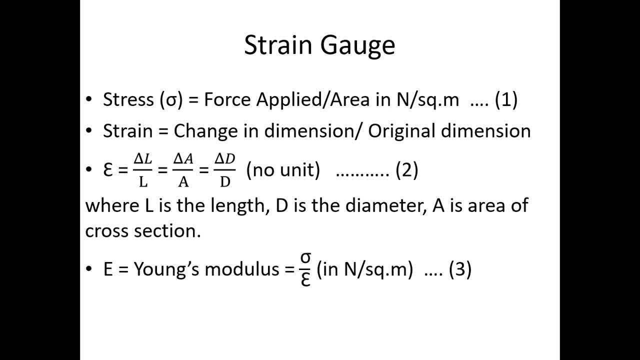 that is normally called as the strain. So strain is nothing but the effect of the stress here. So when you stress the material then there must be strain here, and the strain is indicated by epsilon. Epsilon is equal to del L divided by L. 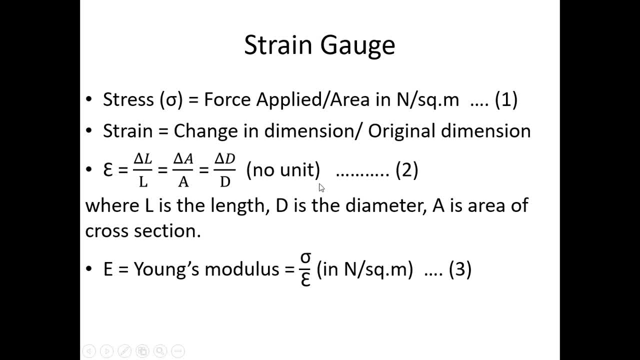 It is also called del A by A or maybe del D by A. okay, There is no unit, because it is all ratio. What is del L by L? It is either you can reflect, you know the strain in the form, in the, you know along the 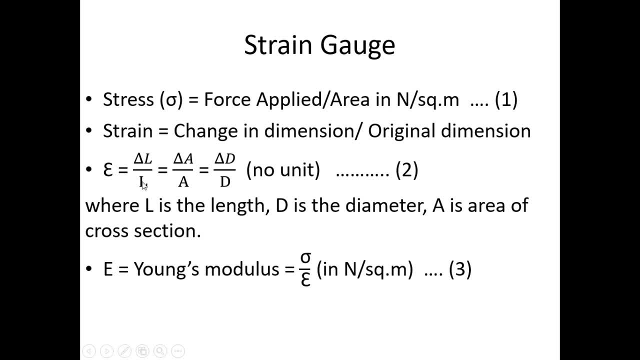 length. So that is why change in length to the original length, or could be change in the area to the original area, or could be change in diameter, you know, depending, you know, with respect to the original diameter. right Now there is also another term which is a constant for a material called Young's modulus. 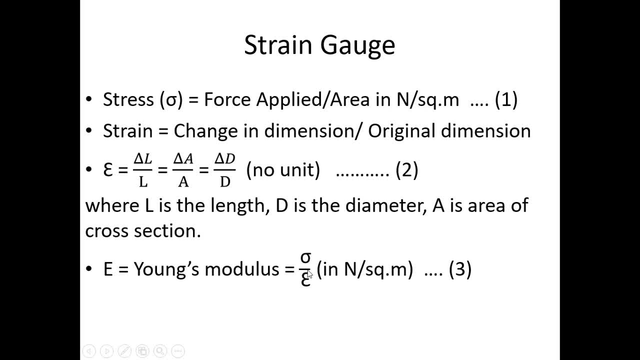 and the ratio of, you know, stress to strain, The ratio of stress to strain, normally called as the Young's modulus. okay, So these are the basic understanding of this material, Thank you. So this is the strain gauge and you know, with this, you know, we will discuss about you know. 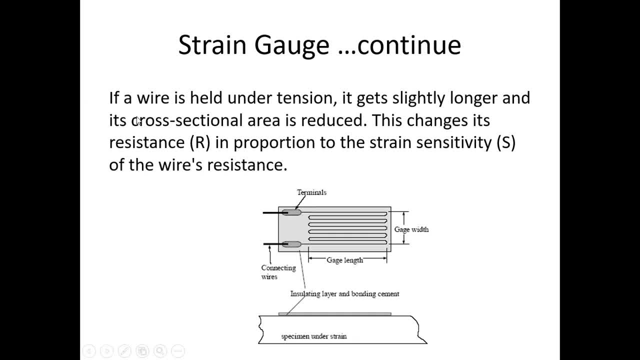 how a strain gauge works. So basically, it is a tiny wire which is held under tension. It gets slightly longer and its cross sectional area is also going to be reduced right. This change in resistance is proportional to the strain or the sensitivity of the wire. 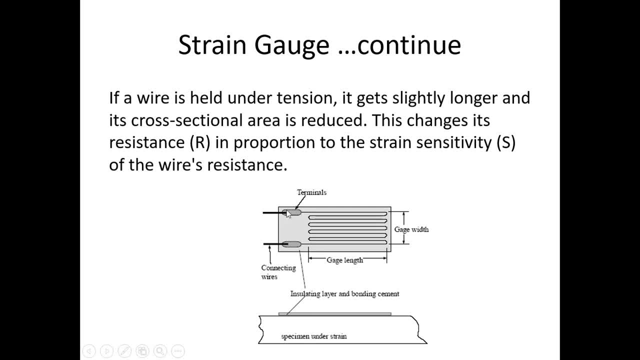 resistance. So what is the basic construction? you know, you can find that there are. this is the strain gauge. There is a tiny, very tiny, you know, wire is, you know, connected between two terminals and normally this particular device or the sensor is attached to a specimen under strain. 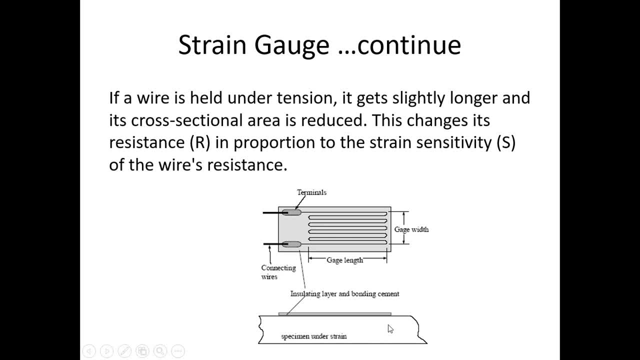 So what happens when this particular specimen is strained or you apply some stress on what is going to happen is that, along with this particular material or the specimen, this is going to be strained or this is going to be stretched, or you will find some changes in the dimensions you know. it could be in the length, or can be radius, etc. 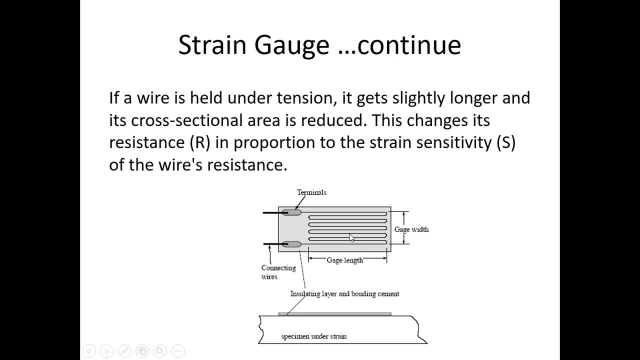 Accordingly, there is some minute change in the resistance value and that resistance value is directly proportional to the change which happens on this particular specimen. So normally that sensitivity of you know, that strain gauge you know, is normally denoted by S and that S is calculated as follows: 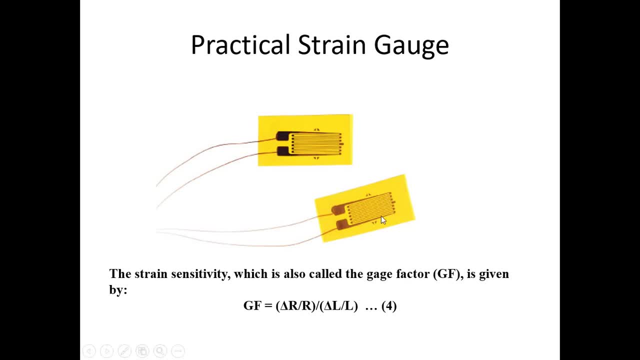 So, before we discuss that, you know this is the physical form of, you know practical form of strain gauge and the strain sensitivity, which is also called the gauge factor. This is the two terminologies: either is strain sensitivity, Strain sensitivity or the gauge factor, and the gauge factor is given by del R divided. 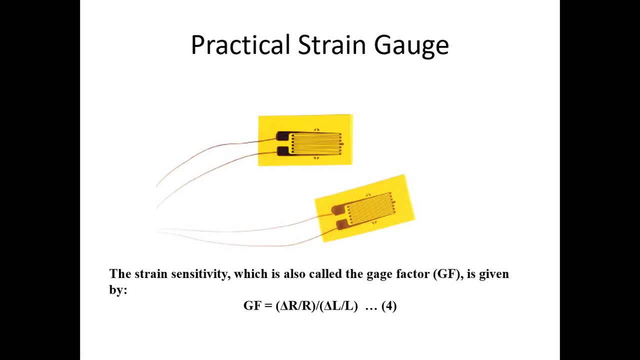 by R, the whole divided by del L by L. So this is basically the numerator indicate change in resistance to the original resistance, which is a unit less quantity, and the denominator is del L by L, which is nothing but changing lengths to the original length. So they are. you know, both are ratios and that is why the gauge factor normally is a unit. 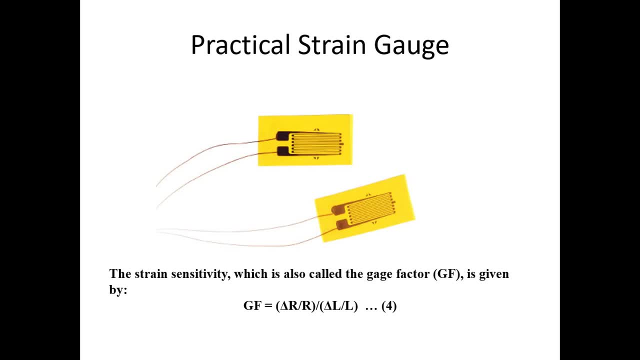 less quantity Now the. as such, you can see that. you can see that there is a change in the resistance and, as such, we saw the strain gauge and the output will be. you know, output will be, change in resistance, while the input is like what the corresponding strain. 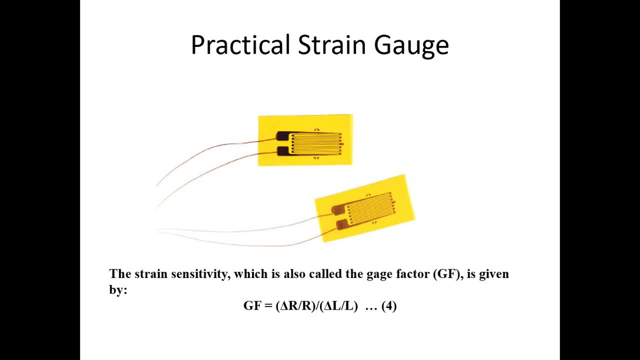 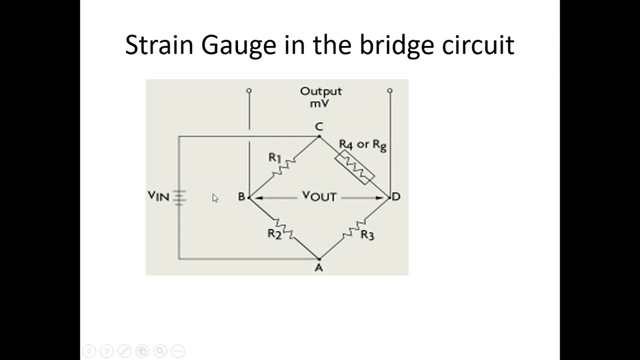 Now, in most of the practical cases we want this change in resistance to be reflected as output voltage. So in such cases, you know we can connect. you know the strain gauge is part of a circuit normally we call as a bridge circuit. So here you can find there is a four arm bridge here and in this bridge, you know there is. 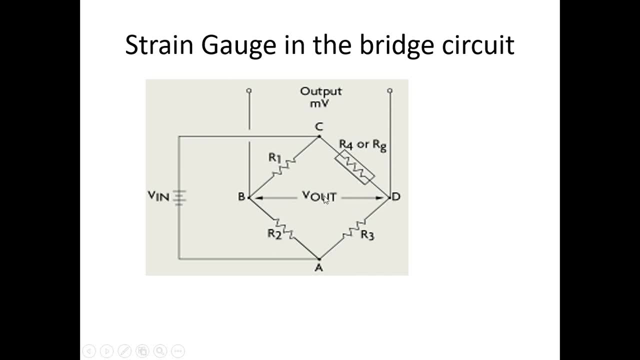 you know, one of the resistance is, you know, acting as the strain gauge here. So what is going to happen when the bridge is balanced? you know, perfectly balanced, then you will get, you know, zero volt across the output here. But if any reason, if you know, out of these four resistors, one resistor is the strain. 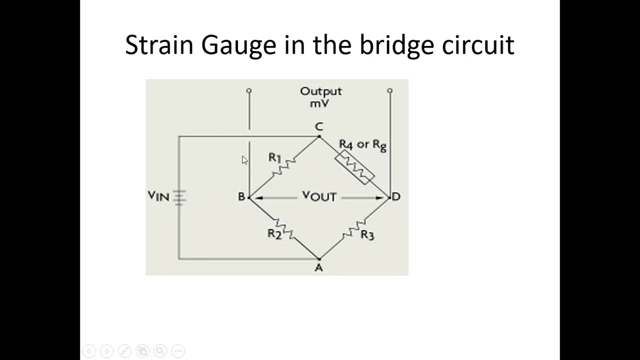 gauge and others are the known fixed value resistors. If you know one of the resistor, which is the- you know strain gauge resistor is changes because of the strain applied, then you will find some change in the output and that output change is directly proportional to the change which happens from this particular strain. 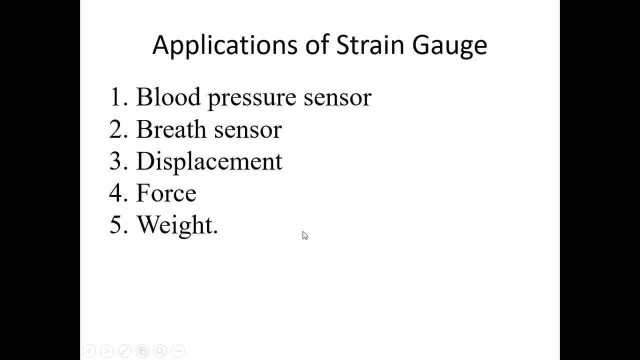 gauge. Now there are many applications for the strain gauge in the practical field and one of such application is the blood pressure sensor. So in blood pressure sensor the change, minute change which happens in the blood vessels, that can be easily measured by using the strain gauge. 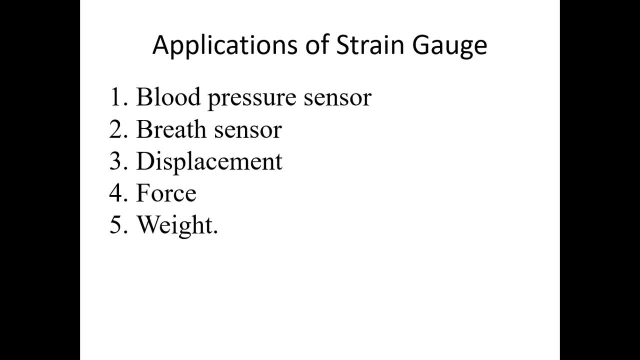 Same way, you can also use the strain gauge for the breath sensor. It can be used for displacement sensors, force sensors, weight sensors, etc. There are many applications for the strain gauge in the practical- you know practical- field. Next, we are talking about the temperature sensor. 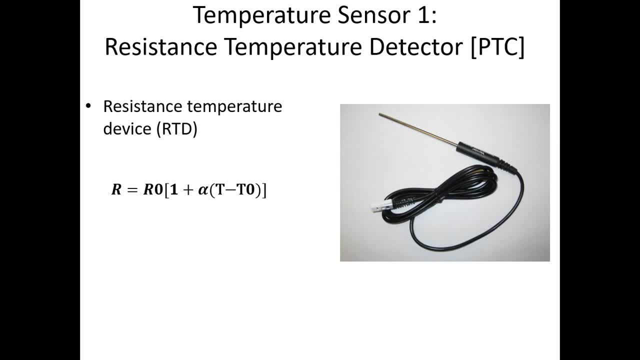 There are different type of temperature sensors are available in the market and one of the common type of sensors normally is the resistance temperature detector. It also belongs to a category of PTC, you know, because if you are using metal as temperature detecting material, then the corresponding change of resistance with respect to the resistance 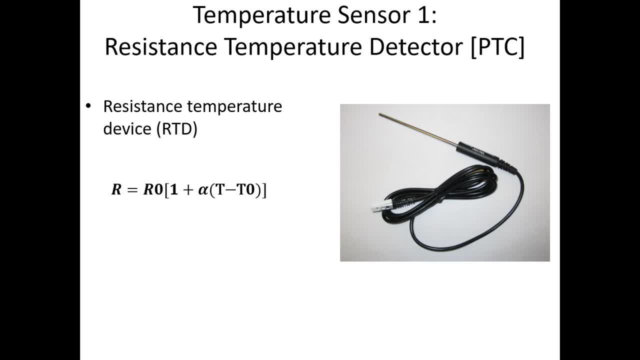 to the temperature, which would be a positive temperature. So that is why these type of sensors is also called PTC- positive temperature coefficient of resistance. And the resistance of a metal that can be calculated by the equation R is equal to R0 into 1 plus alpha, into T minus T0. 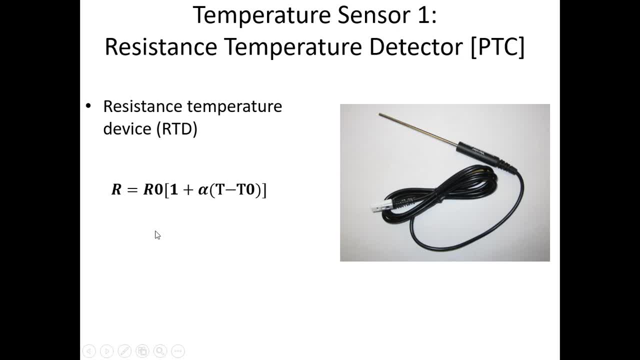 So where R0 is the resistance to standard, you know temperature, or maybe 0, you know 0 temperature, 0 degree centigrade or any other reference temperature, And 1 plus alpha means it is a constant temperature coefficient of resistance, And T and T0,. T is actually the measured temperature and the R0 means the reference temperature. 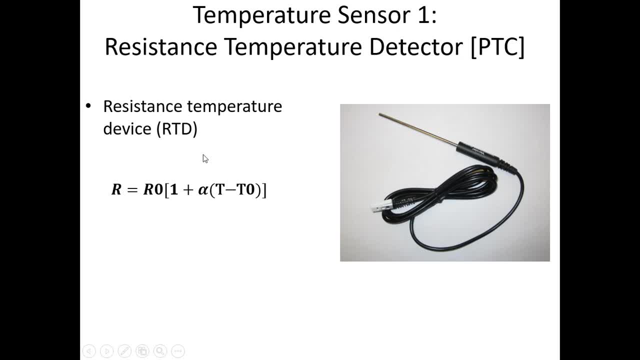 So this particular reading is based on a reference temperature. So, for example, if you are considering 10 degree is the reference temperature, then this is supposed to be 10 degree. Then the actual temperature could be 20 degree. So in this case we will have, you know, 20 minus 10, that will be the temperature difference. 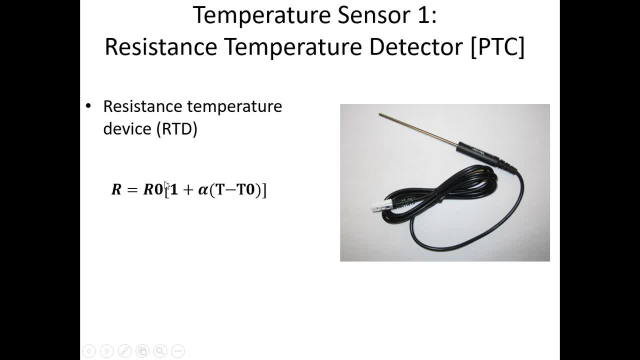 that is multiplied by a constant called alpha, Then that is going to, you know, add 1. Multiply by the value of R0.. R0 is nothing but the resistance which is corresponds to the reference point here. Okay, Now this device can be used to measure the output. 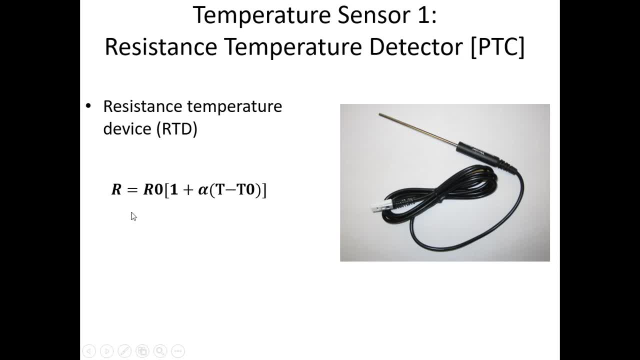 But here again the output is in the form of resistance Right. So in order to measure, this is on a digital device, definitely, you know this output reading we have to transform into, you know, current signal or voltage signal and by using some kind of, you know, associated circuits here. 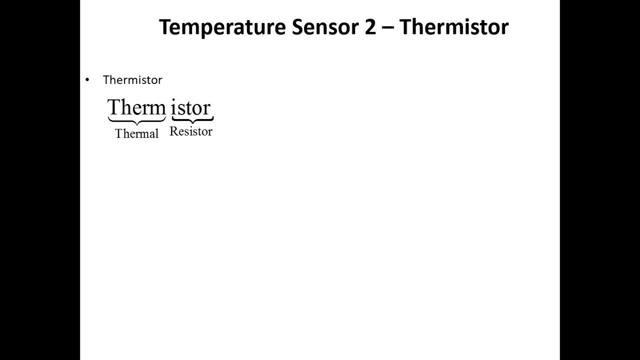 There is another type of sensor. This temperature sensor is called the thermistor And from the name itself is clear that you know it is the two terms. One is called therm. Therm means the thermal or the temperature, And the remaining ester stands for the resistor. here. 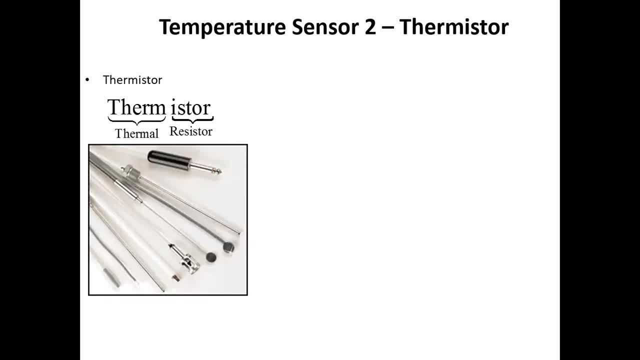 So it is nothing but a thermal resistor And they are also very commonly used in our field And there are different type of sensors. you know the thermistors are available in the market. Okay, So now R0.. The thermal thermistor resistance of a thermistor that can be calculated by using the relation. 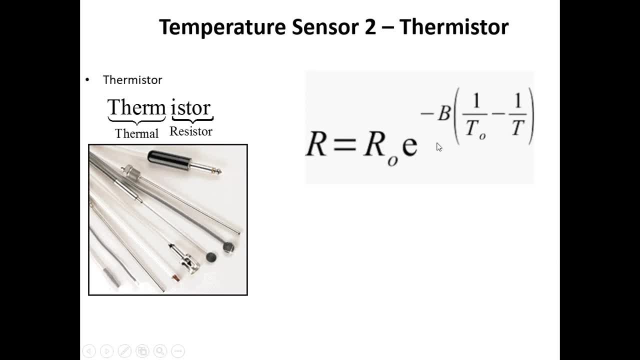 R equal to R0 into e, to the power minus b or beta into 1 by t o minus 1 by t. So here R0. as we have discussed already, it is a standard, you know reference temperature. I mean the resistance at standard temperature or any other you know known temperature that 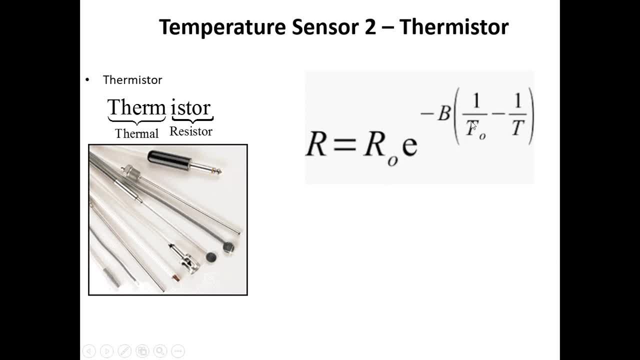 is R0.. In this example, R0 is, you know, with the reference to R0.. Okay, R0 is the reference to T0.. Beta is a factor that is a constant, you know, for a specific thermistor, And T is the. you know the temperature that, you know the actual temperature that we want. 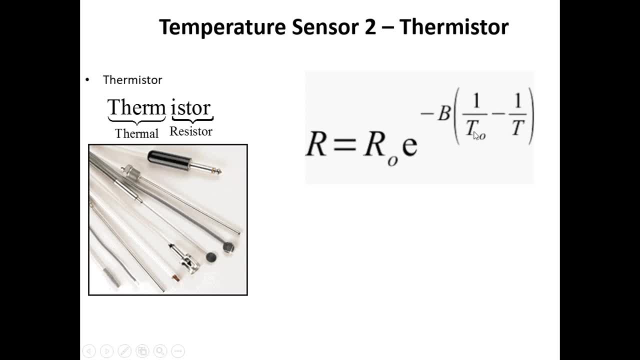 to measure it. Okay, So T0 is the reference temperature and T is the actual temperature, And the change is going to reflect on the resistance here. Now, depending upon the response, like whether they are responding positively or negatively, we have two type of sensors available in the market. 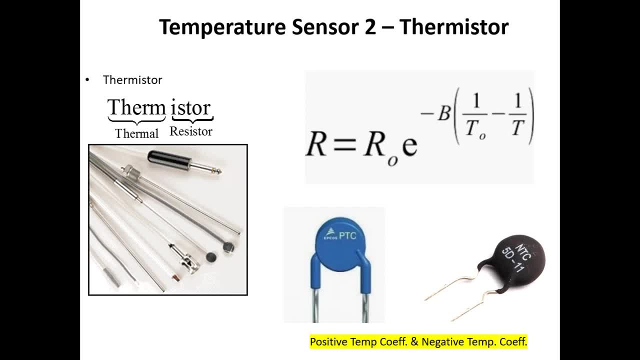 Which are PTC sensors and NTC sensors, The positive temperature coefficient sensors and negative temperature coefficient sensors. Okay, The only difference both of them are one is, you know, changing with respect to positive. So as the temperature increases, the temperature is also increased. 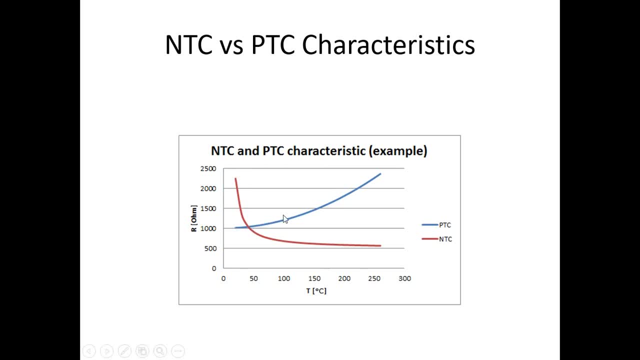 So you can see here, in the case of PTC, as the temperature is increases, the resistance values also increases, Right, Whereas in the case of NTC it has got a very high resistance in the beginning when the temperature is very low. As the temperature increases, the resistance values also increases. 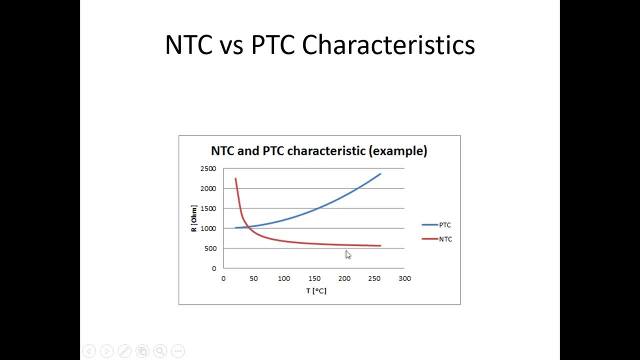 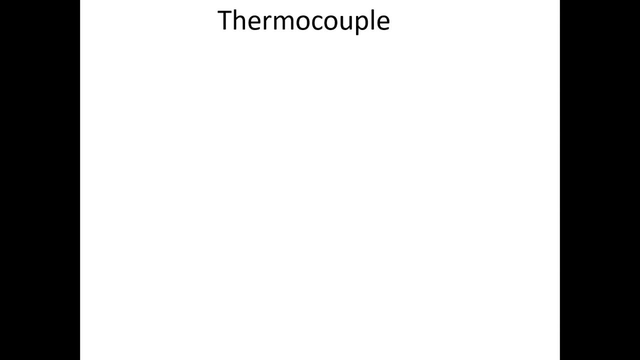 Right, As the temperature increases, the resistance drops. So there are practical applications, for you know these type of NTC and PTC, you know thermistors. Next device is called the thermocouple. So thermocouple is basically is a couple of two different substances, or two different. 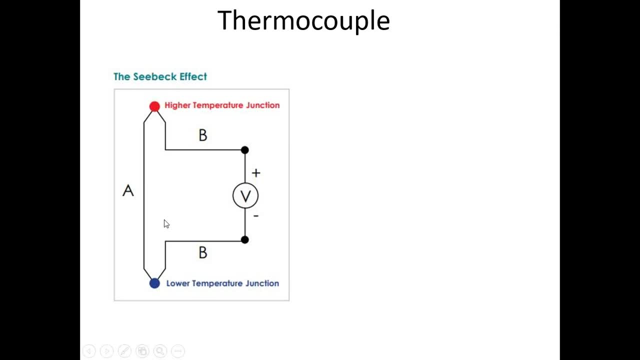 materials here. Okay, So what we can see here, you know we have using two different material. One is A, A material A And other metal is like B, So there are two different metals, Okay. So one is like copper and could be, one is, like you know, constant an. 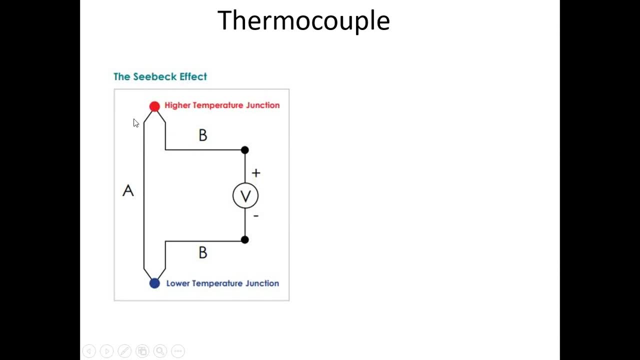 Okay, So either copper, constant an or any other, you know combinations where we would use one element. here I mean one material, metal A, and another metal B, And we have got two temperature here. One is called the lower temperature, is sometimes is also called the reference temperature. 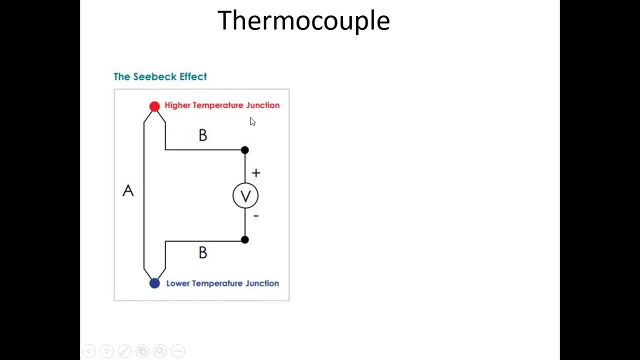 And the other temperature is called the higher temperature, which is supposed to be measured. Because of this temperature difference, you know, then it is amazing to note that there is a potential that is generated, And that is first, you know, you know, found by Seebeck. 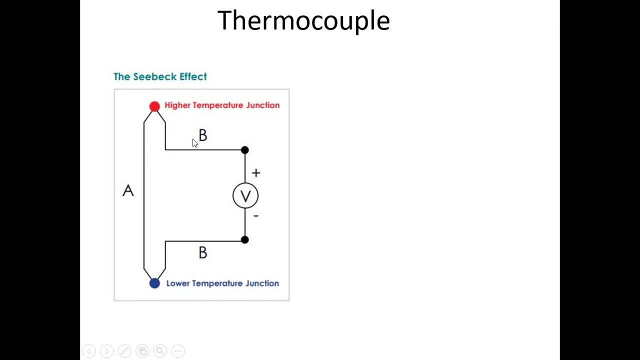 So that is why it is called Seebeck. you know effect: Okay. Now, according to the Seebeck, when there is a difference in the temperature and because of some Seebeck coefficient, you know, you find some. you know output voltage here. Okay, Now how we are going to use this device for the measurement. 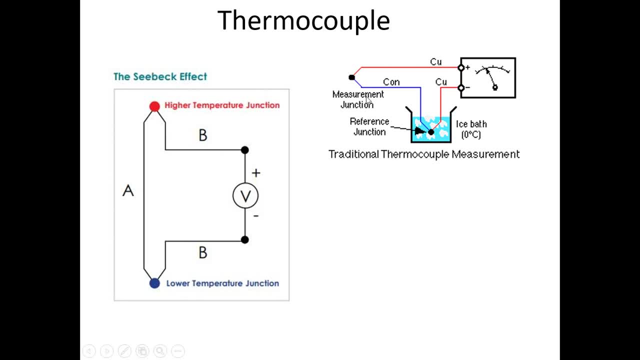 So, for example, if you are trying to measure the temperature of inside a furnace or some very high temperature That is to be measured, Then here we are using the, you know, copper constant, an as the basic material And one junction, one point you know, because we have got two junctions here, blue color. 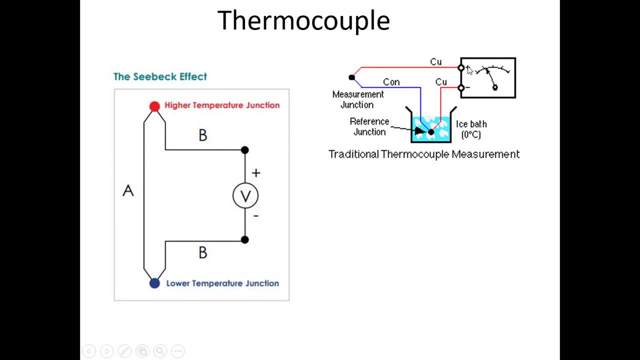 indicate the constant an and the red color indicate the copper. So one of such joint. you know we are going to keep as reference temperature by using some kind of ice bath, by keeping the temperature is somewhere around zero degree centigrade, Whereas the other temperature- other point- we want to keep at the temperature you know. 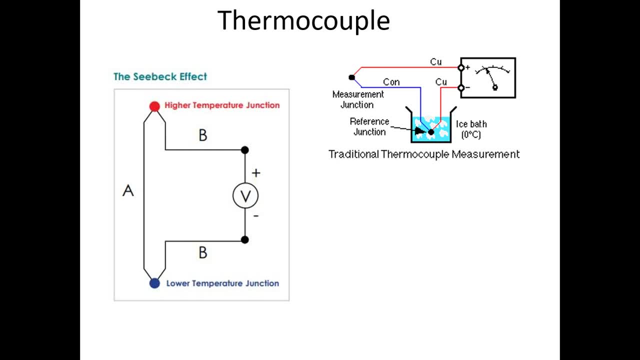 Of the sample or the temperature that is to be measured. Now, because of this temperature difference, you will find some output reading here, And that output reading is directly proportion to what I call the temperature difference. Now, this is a practical device. you may find it in the market. 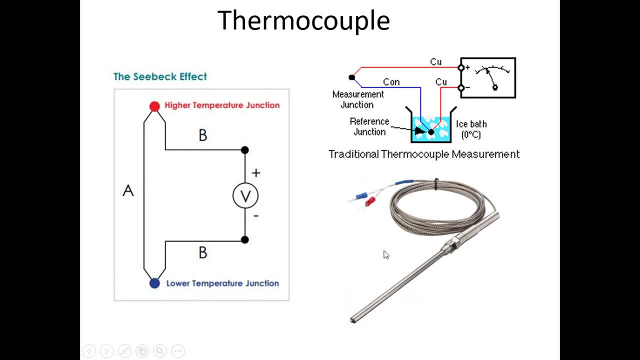 So you know it can be used for measuring very high temperature here. Okay, Now the basic equation is: the output voltage is equal to a factor S, which is the Seebeck factor, multiplied by Tx minus T reference. here, Tx is the output, T is the temperature that is to be measured. 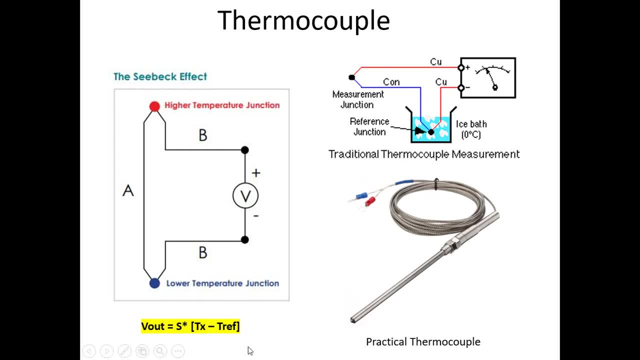 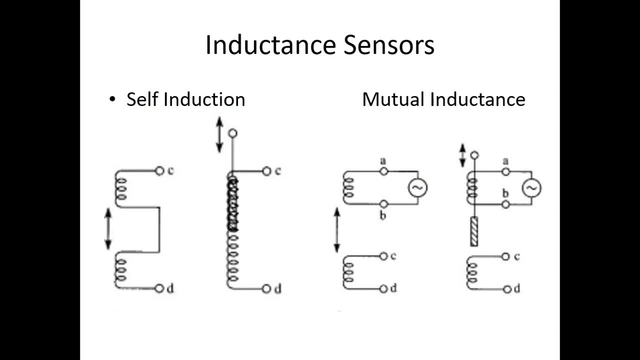 And T reference is the reference temperature. Okay, It could be. you know, sometimes it can be zero degrees centigrade. So now we are talking about the inductance sensors. Here again we said you know, the physical quantity that is being measured is going to change. 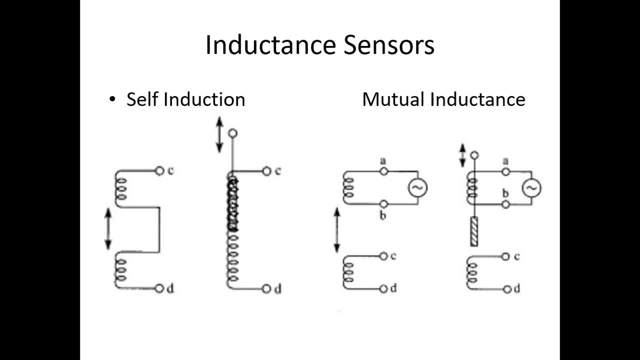 the inductance of the material And the inductance are different types. The inductance are classified into self inductance and you know mutual inductance here. So from the graph it can clearly you know clear that there are two set of coils are here is: 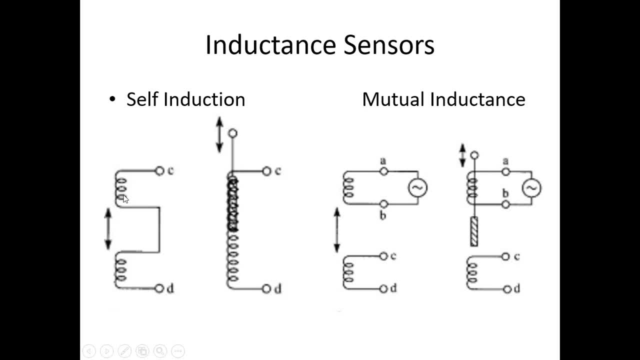 connected. So if we are interested, you know- I mean we have got one set of coils and that can be. you know, you know design in this particular pattern And you can find that there is a metallic core is inside. you know this part, you know it is nothing but the metallic core. 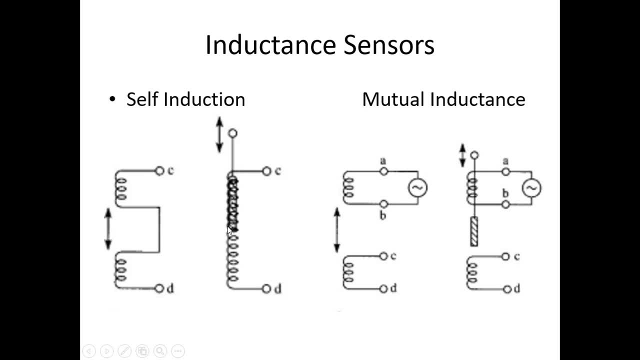 So by moving this metallic core up and down, is it possible, you know, to generate some EMFs here. And what we have found? that the inductance of the coil or the voltage induced in a coil, that is depending upon the position of, and you know, the particular core here. 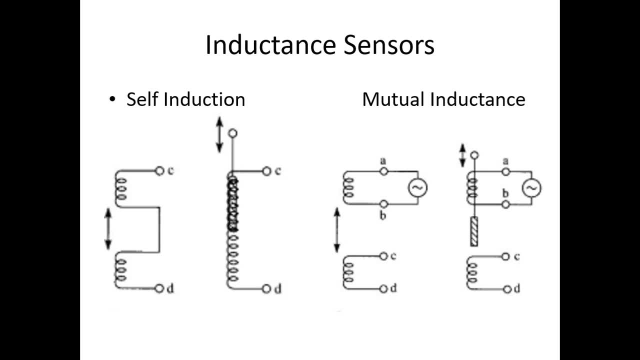 And also it is also depend upon the speed or the velocity of the motion, etc. So there are many factors which also, depending upon the number of turns here, it depend upon the size of the core, depend upon the magnetic permeability and so on and so forth. 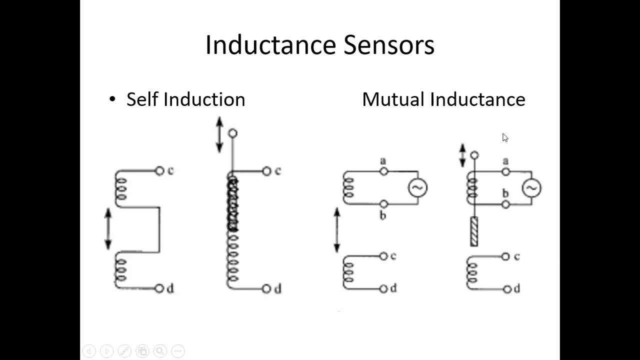 Now, another type of sensors is called the mutual inductance. So here we have using a single set of coil here, But here we are using two set of coil. And what we are trying to do, you know, we are going to make a change in the voltage because 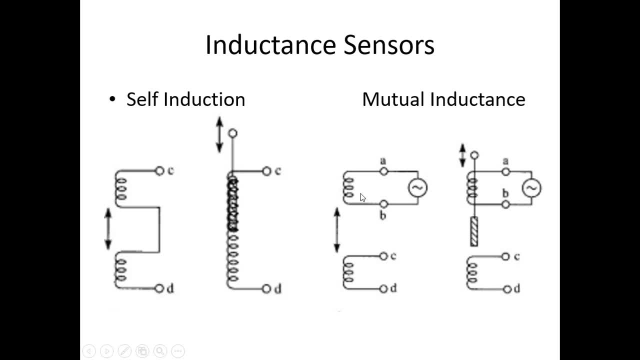 of the change in the voltage happening in another coil. So we are going to make a change in the voltage because of the change in the voltage happening in another coil. So what we can see, we have a set of coil here, AB here one set of coil, and CD is another. 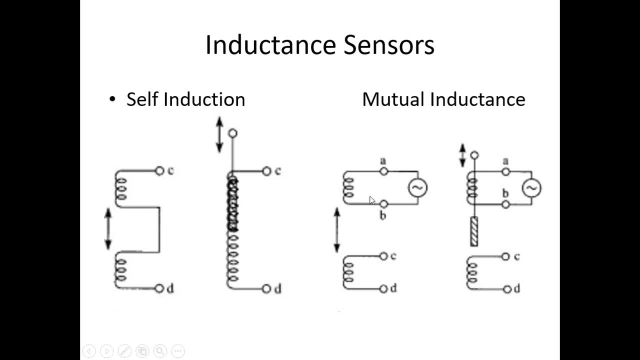 set of coil. We are changing the voltage in this particular coil, which is AB, because of the effect called mutual inductance And since they are, these two coils are situated next to each other. what is going to happen? you know, the change in the first coil will impact or will, you know, introduce some change. 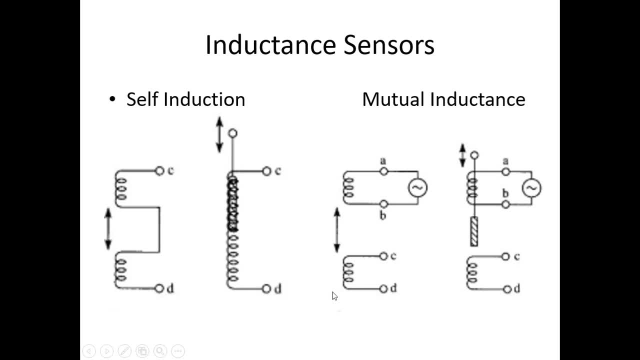 on the, you know in the coil C and D. as a result some voltage will be induced, And So this type of inductance normally we call as the mutual inductance here. So this type of coils that can be used for measuring what you call the linear as well. 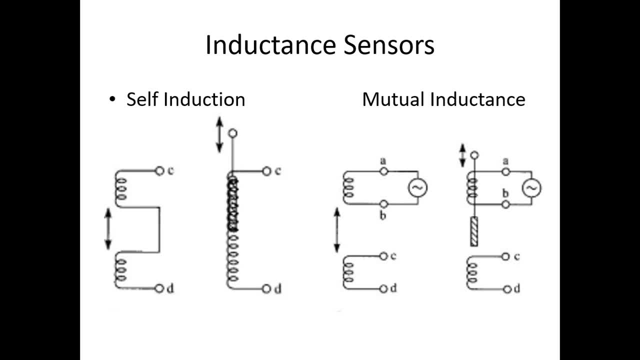 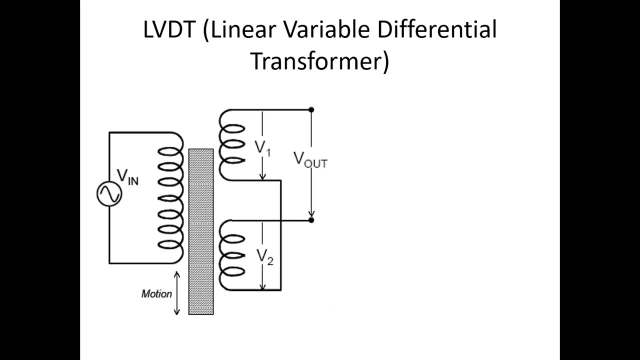 as the you know, angular type of, you know measurements. So, basically, these are the you know sensors that can be transformed, the mechanical vibrations, into electrical signals, And one of such you know the sensor which very, you know, very commonly used, is called the LVDT. 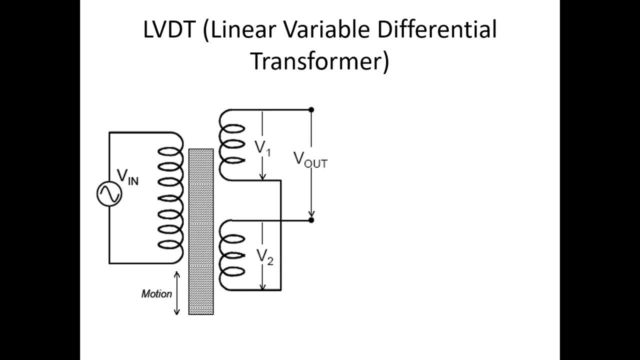 LVDT stands for linear variable differential transformer. So what you can see here there are four basic terms: linear, Linear means what is used for linear motion. Variable means you know the output will change. Differential means you can see that there are. you know this is a kind of transformer. 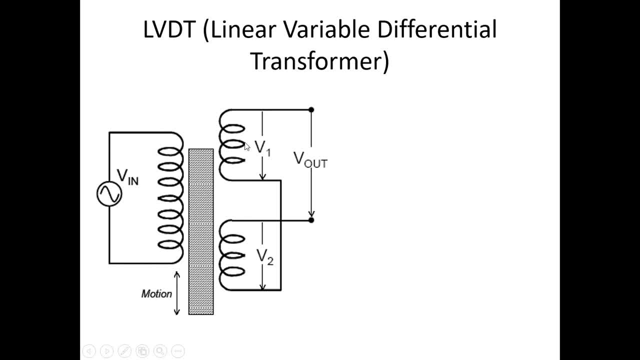 This transformer has got a primary winding and there are two secondary winding. The specialty of this transformer is the transformer core, you know, the core which connect between the primary and secondary, the metallic core That is that, can, you know, move. this is, like you know, a mobile type of what you call core. 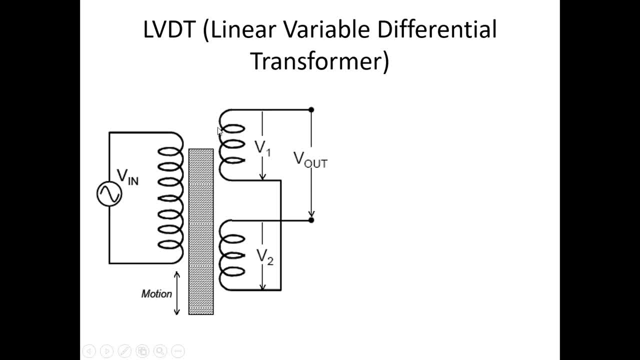 And the output of the secondary is. I mean they are connected in such a way that the output will be always the difference of V1 minus V2. that is why it is called differential, So linear, because of the linear can be used for linear measurement and variable means. 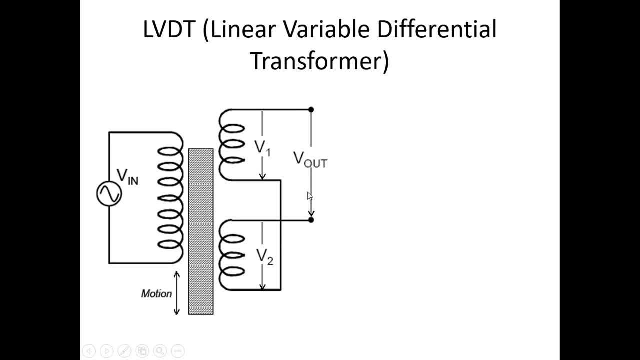 the output will normally change. Differential means the output is normally, you know, the connected Right, In a way that the output will be always a difference, because Vout is equal to V1 minus V2.. Then let us suppose that the coil is exactly located, I mean the core is exactly located. 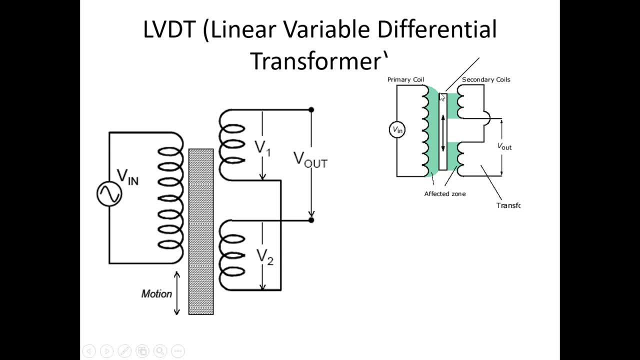 in the middle, I mean exactly in the middle, where it is completely linked with what you call these, both the secondary coils. you know, equally, As a result, what we can find: that in the voltage which is induced in the coil number one and coil number two, exactly same, and the output will give you a zero reading because V1 minus. 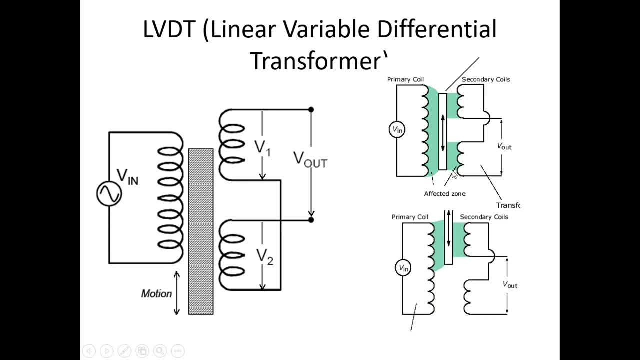 V2 is equal to zero. Now, on the other hand, if you can see in this particular image that you know, this coil is located extreme, you know, just you know, with I mean linked with only the coil, top coil, and it is away from the first coil. as a result, this voltage will be higher, which means in 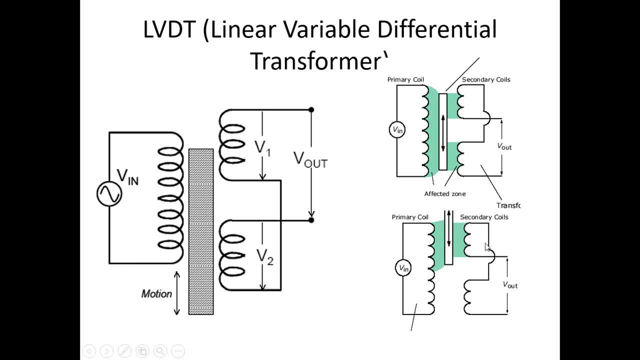 this example, V1 will be higher than V2.. As a result, V1 minus V2 will give you some number and that number will be proportional to you know the position of the coil here. So by this method and on the other hand, if you are moving, this is to the other side. 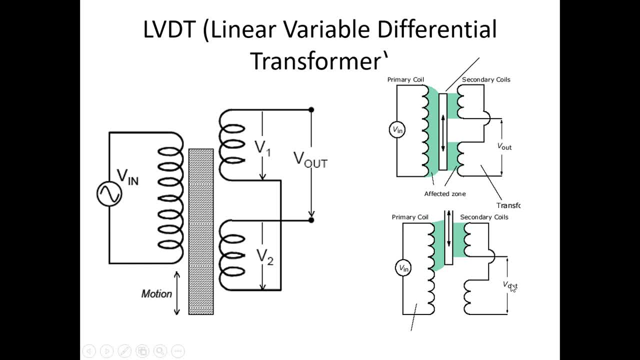 All right, we will have an opposite nature here. So by this way, any voltage, any position of what you call the core will give you a corresponding change in the output in the form of either positive or negative voltage. okay, So this particular device is used in many applications where you can measure the vibrations. 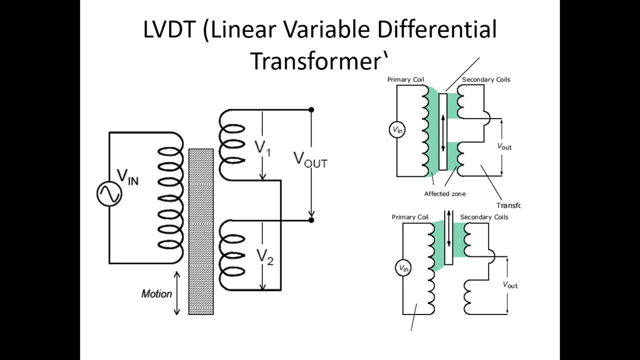 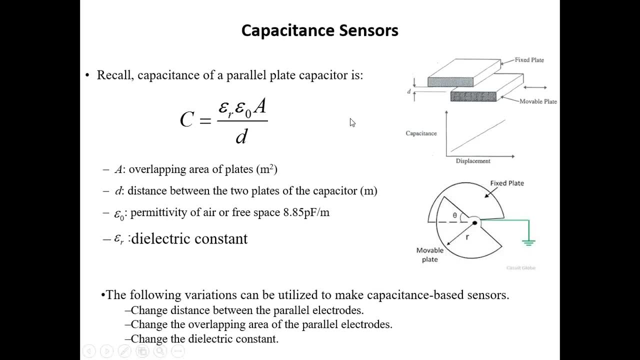 you can measure the displacement etc. very accurately. And the next type of sensor is the capacitive sensors and from the basic parallel plate capacitor rule, see the capacitance of a parallel plate capacitor is calculated by the equation: epsilon r, epsilon 0, a over d, where epsilon r is the relative, you know the permittivity. 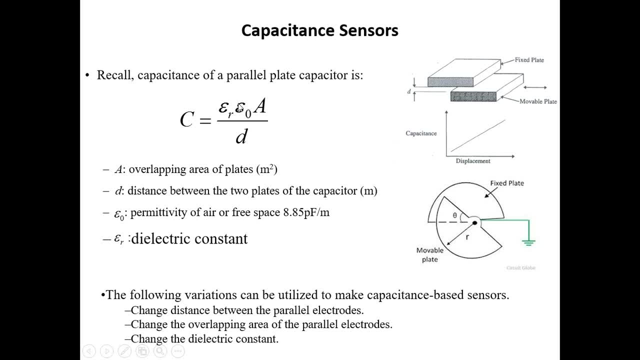 of the medium and epsilon 0 is the absolute permittivity which is normally constant. it is 8.85, you know, picofarad per meter. a is the area of the plate in this particular example. if you look at this is the area. then if you multiply it by the length, by breadth, you will.